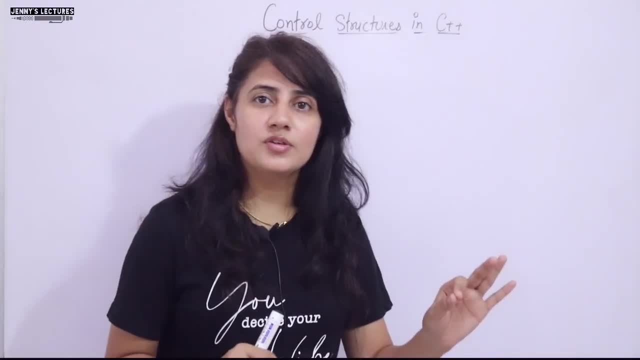 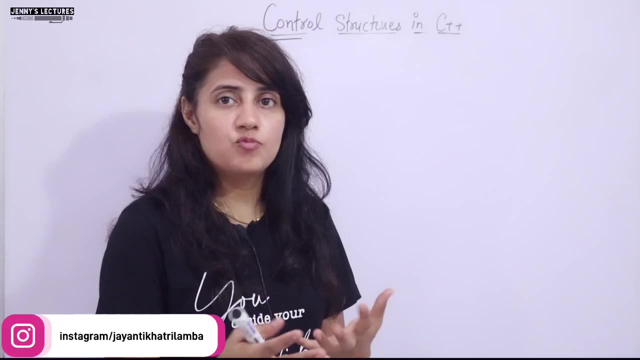 So in the series of learning C++ programming language, in the previous video we have discussed operator precedence and associativity. We have discussed all the type of operators and then operator precedence and associativity, with two or three examples With the help of program I have. 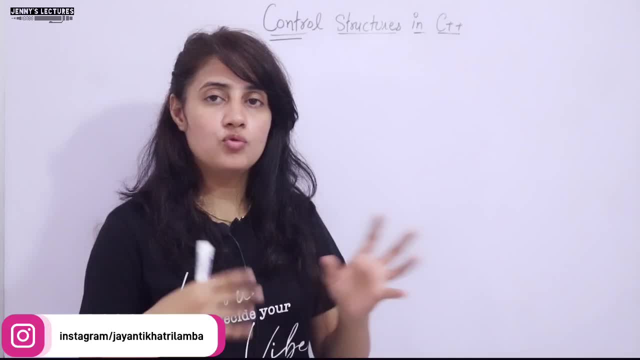 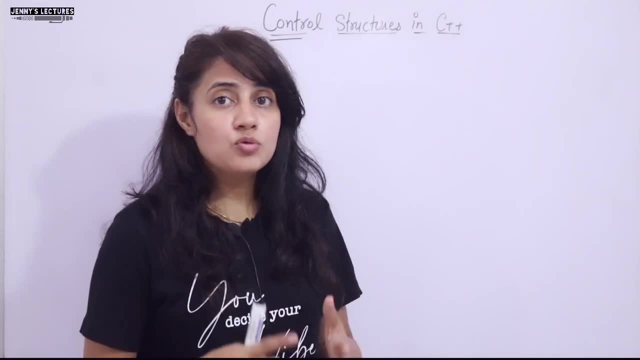 shown you everything about precedence and associativity Right, How to apply precedence and associativity and when to use these things. We have discussed this thing Now in this video. from this video I am going to start control structures in C++. First, the basic: what is? 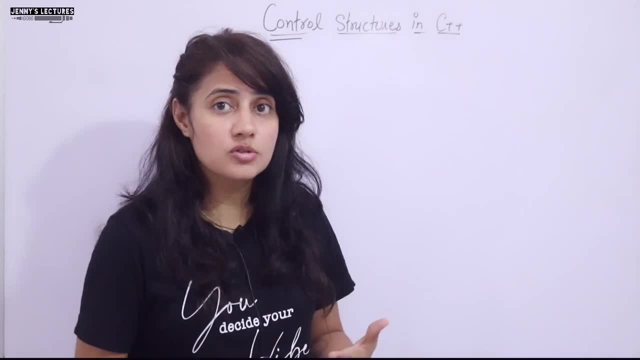 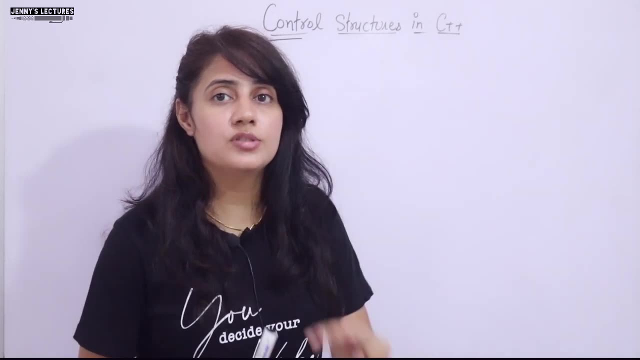 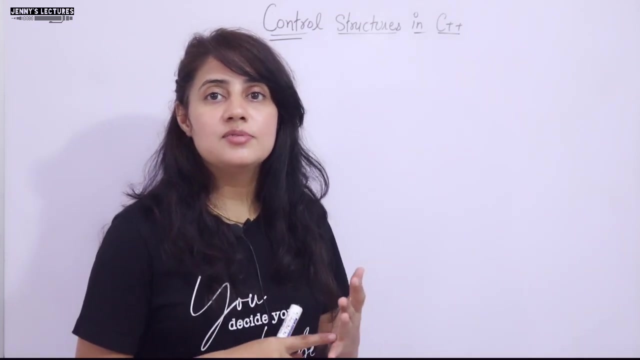 control structure, why we use it, different types of control structure, and then, in detail, we will discuss one by one Right. So basically there are three basic type of control structure: Sequential, selection and iteration. Right Sequential means, as the name suggests, 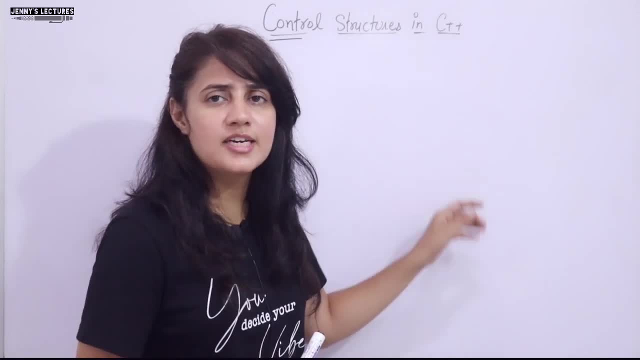 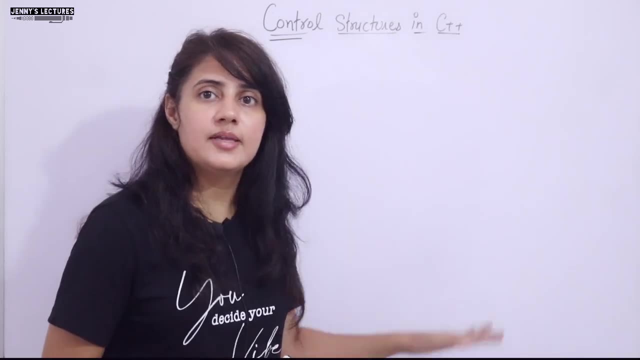 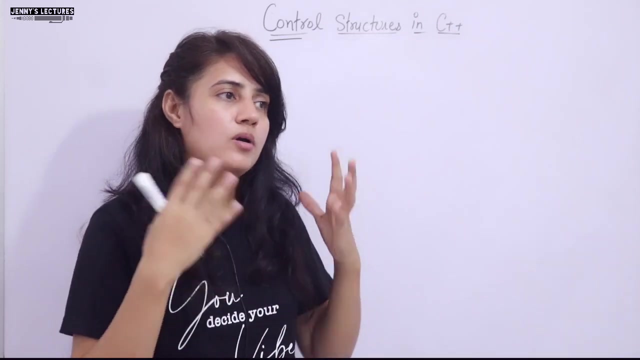 Whatever statements you have written in the program, the statement would be executed one line by line Right In a sequence, Whenever they appear they exist in a sequence Right, So in a sequence, whenever they appear they exist in a sequence Like the control will start execution from the main. If suppose I write a program to print sum of 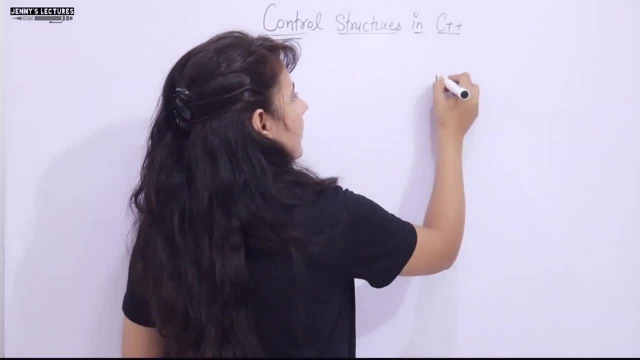 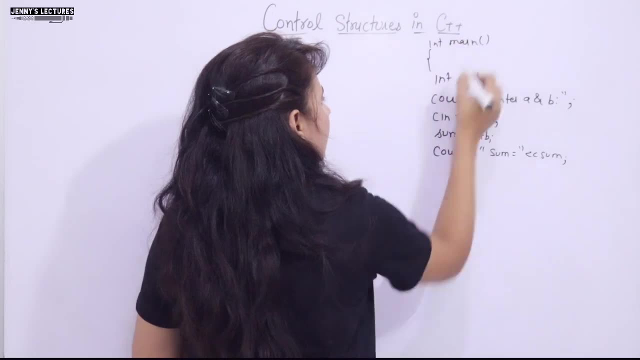 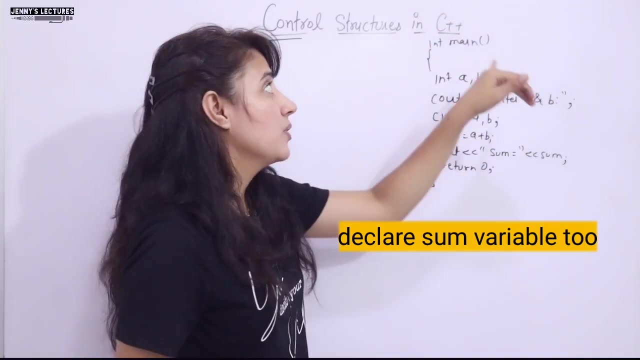 two numbers Right. So simply in main we take two numbers like int a, b, then cout. This is simple program to calculate sum of two numbers. Obviously you can write down that header file using namespace. std. Program will start executing from the main function. then this line will be executed: 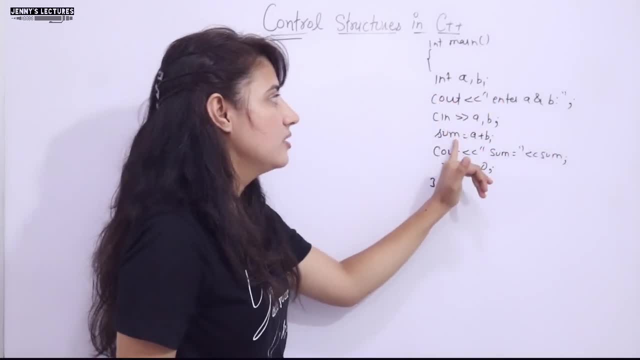 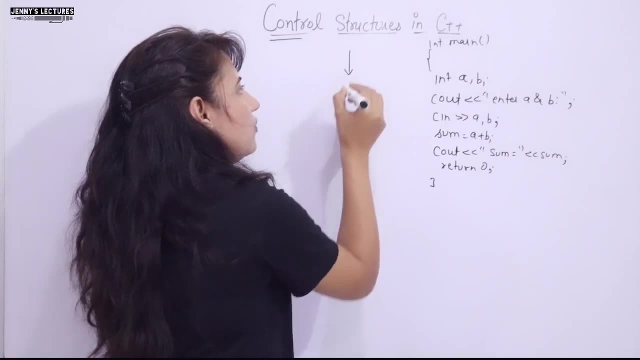 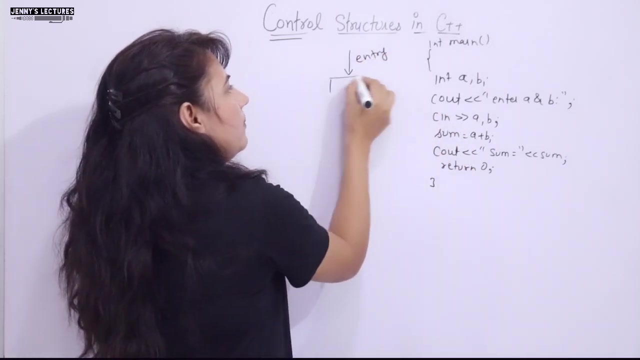 int a and b, then cout, enter value of a and b, then c in, then sum would be calculated, then sum would be printed and returns 0.. This is simple sequence. So simply we will. you can say with a flow chart how you can show enter into the program. Entry point is main function, One by one statement. 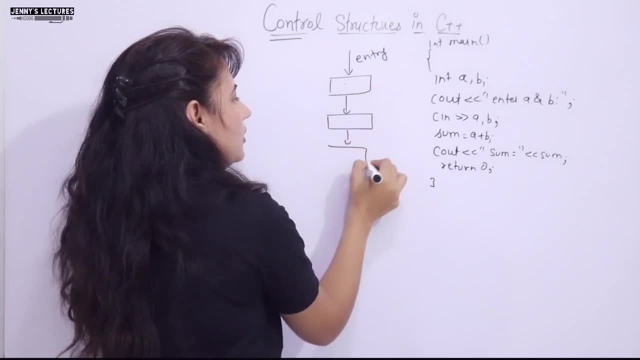 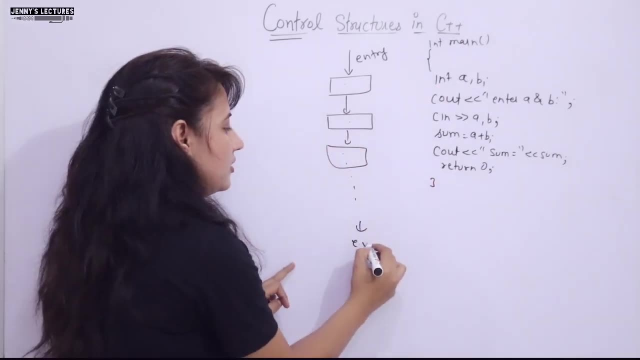 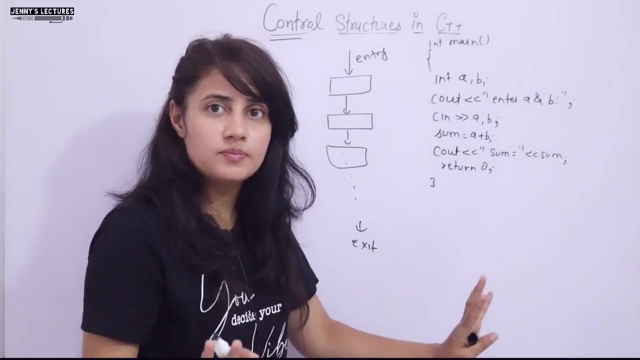 would be executed: Statement 1,, statement 2,, statement 3,, statement 4.. How many statements are there in a sequence? all the statements would be executed line by line and at last exit from the program. This is, by default control structure of a program. By default Right. Next comes 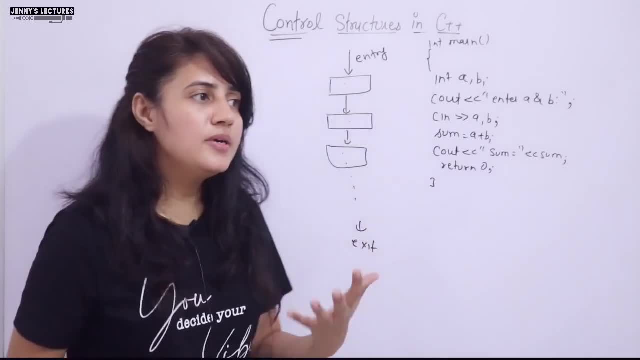 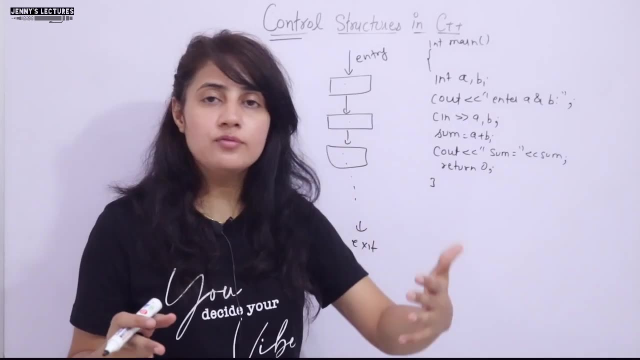 to selection control structures Now. selection means you have to select something based on some condition. You have to decide something Right. You have two choices. You have choices Right, Suppose you have choice. you have two things: coffee or tea. Now you have choice. 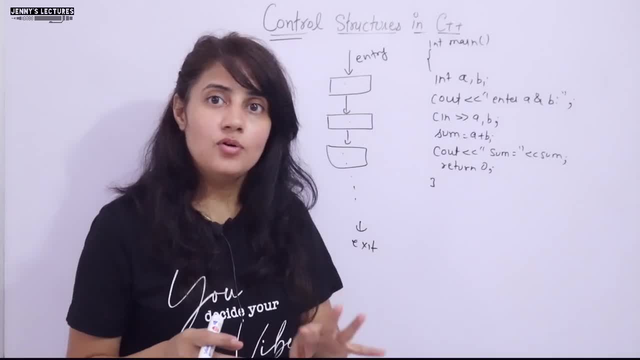 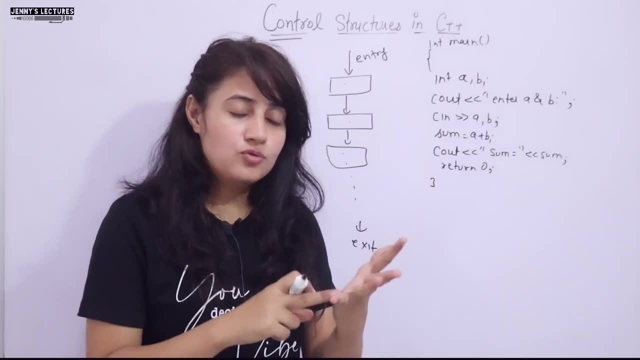 which one you want to drink: coffee or tea, Right Switch. Now you have two choices: How? If only tea is available, you don't have any choice and you will drink tea, right, You will have tea. Now you have choice. like you have coffee, you have tea, you have juice, different type. 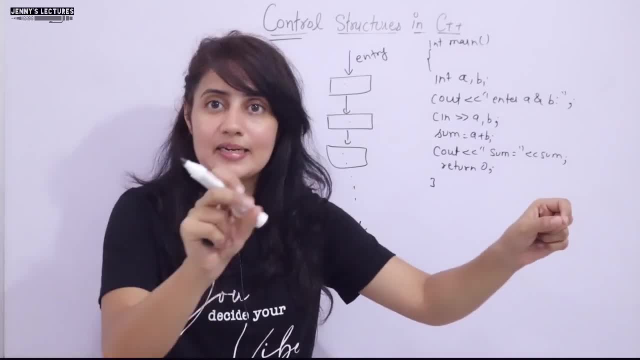 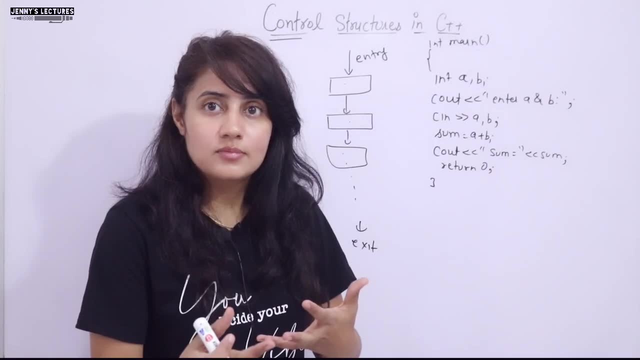 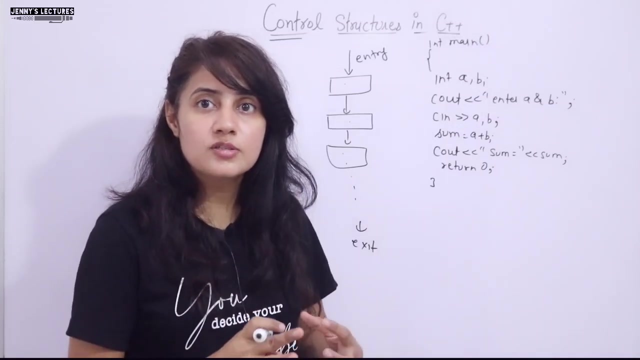 of juice. Now you have choices. Now you have to select right Which one you want to have. So this is what selection process, or you have to decide right- Same in program also. we have choices right How you can implement these kind of choices with the help of a program using selection. 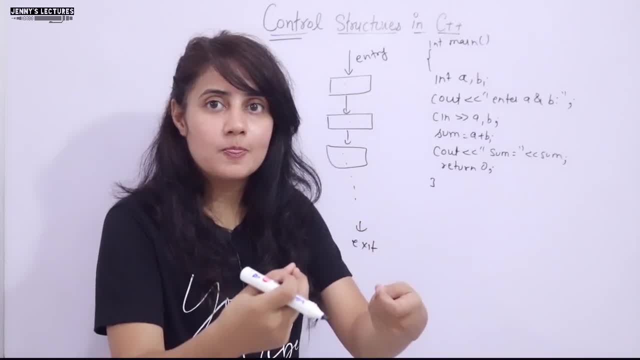 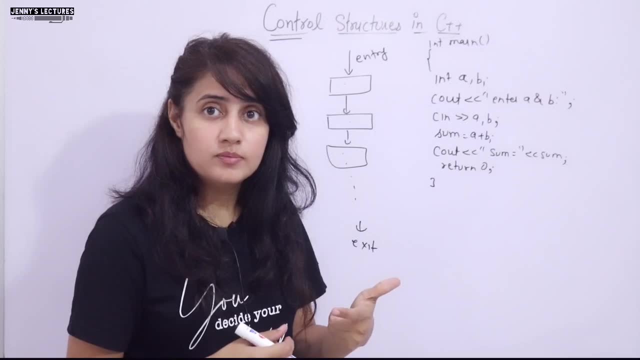 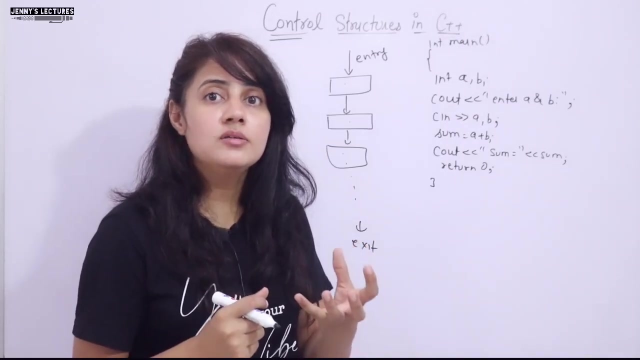 statements, or you can say decision making statements, right. So some statements or a block of statements would be executed based on some condition, whether the condition is true or false. Based on that thing, the statements would be executed right. And that condition can be any expression or any constant value, but the condition should 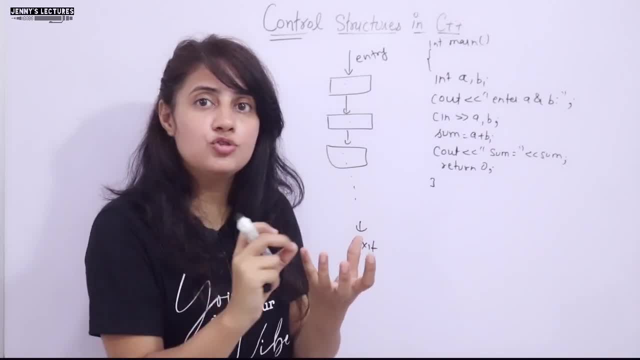 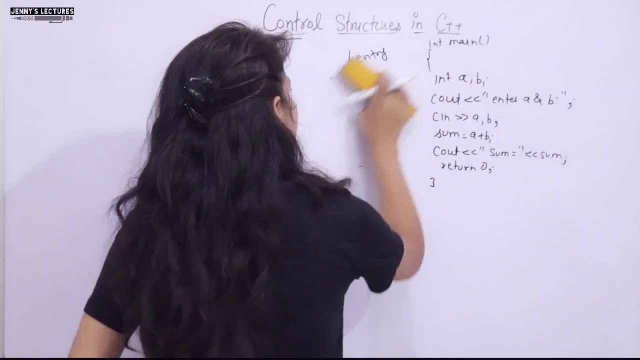 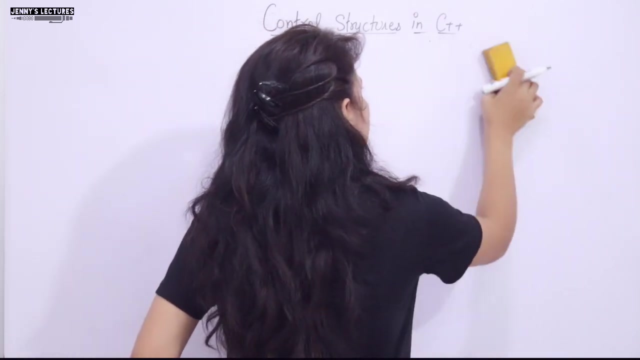 be true, It should be evaluated at last. either true or false, It should be evaluated in a Boolean value, right. So selection in selection, you know, control structure, we have some, you can say, some statements, or those decision making statements you can say, or the selection statement, we 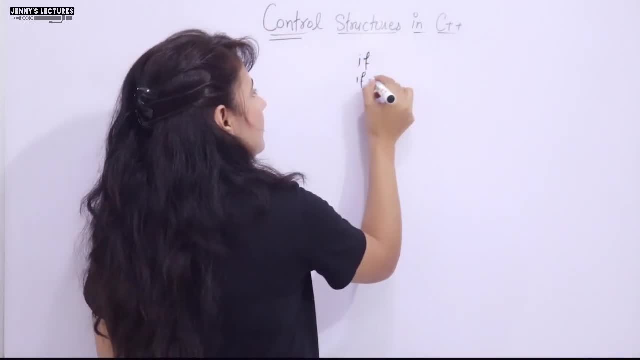 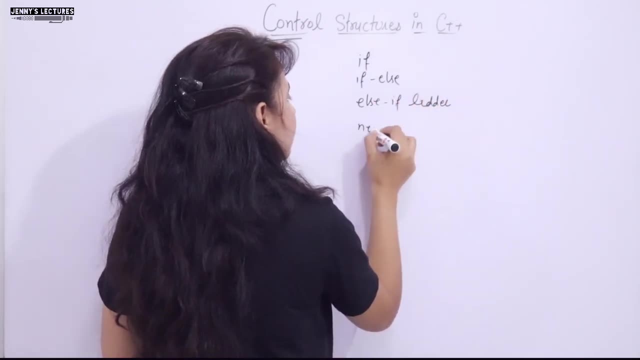 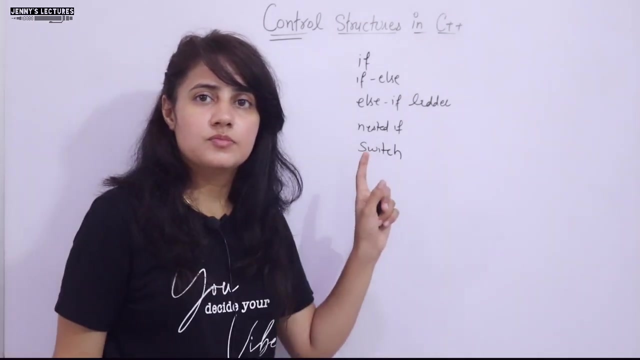 have if, if else, and when we have else, if letter, then we have next, if letter, then we have nested. if, then we have switch. right, These are selection statements, right? So these comes under those selection control statements. you can say: or selection control. 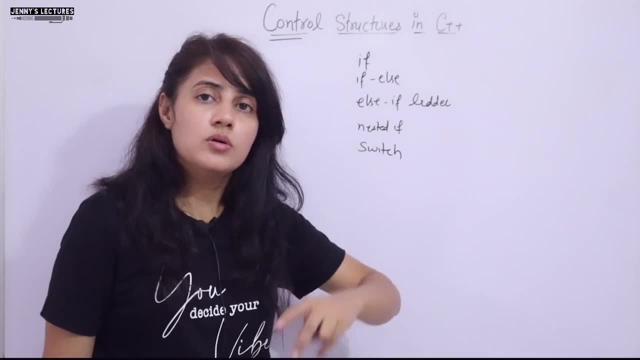 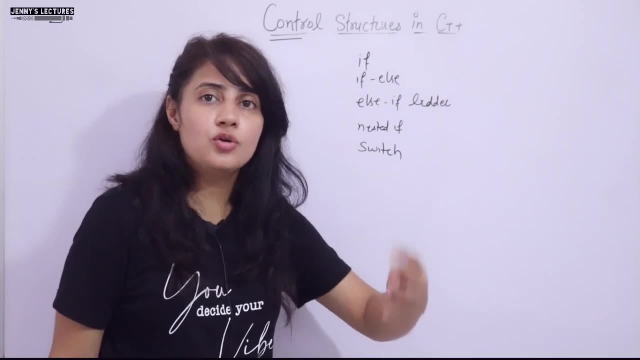 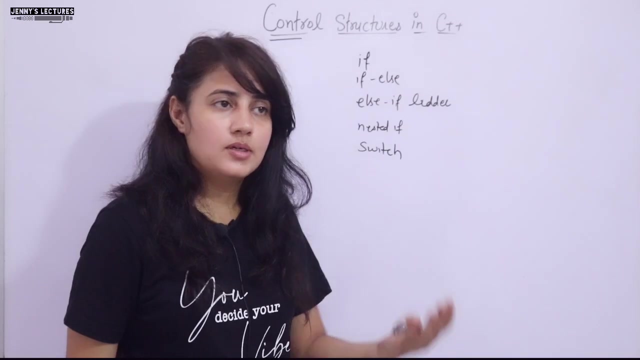 structure right. Third comes to iteration: iteration right. Iteration means repeatedly. we are executing something based on a condition right. Again and again We are doing same thing, right? If you are eating something, then we take one bite of the chapati right? 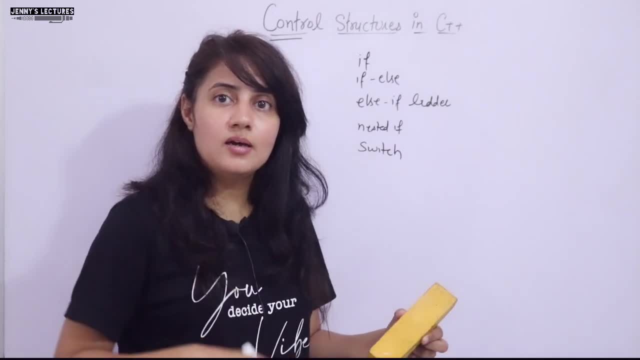 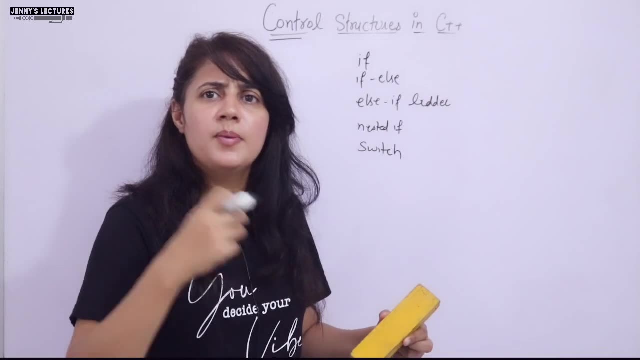 Then we take second bite. The condition is: till our tummy is full, we will eat right. Then one bite, then second bite, third bite. same task we are repeating again and again. We are taking bite right: Chapati with sabji. 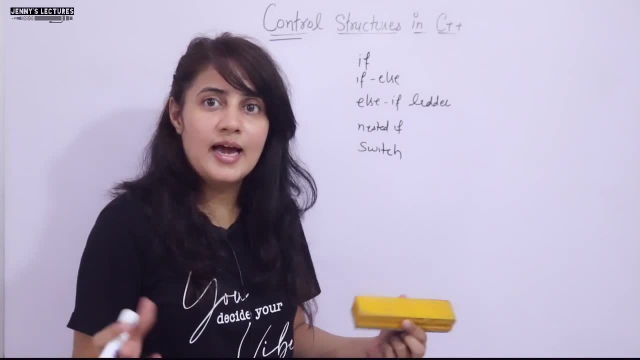 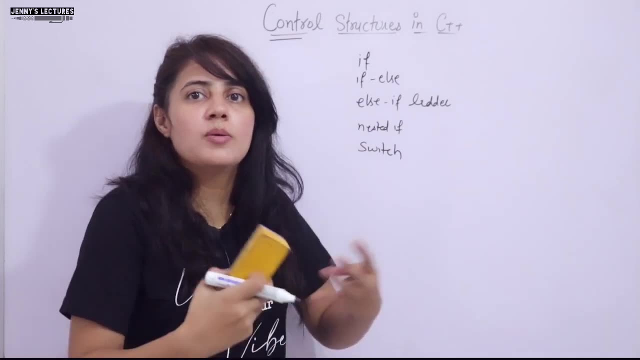 Whenever you are full- your tummy is full- you will stop, And that is the exact condition. So means iterative, means repeating the same steps again And again. right, Based on some condition. right, Like suppose, if you want to print a value from 1 to 10, right. 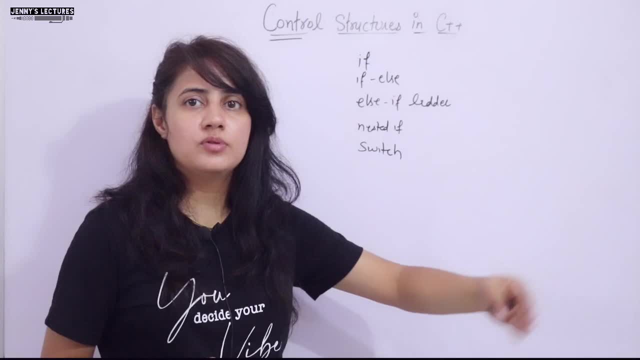 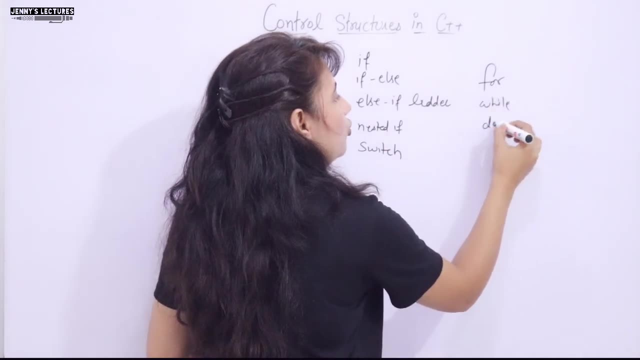 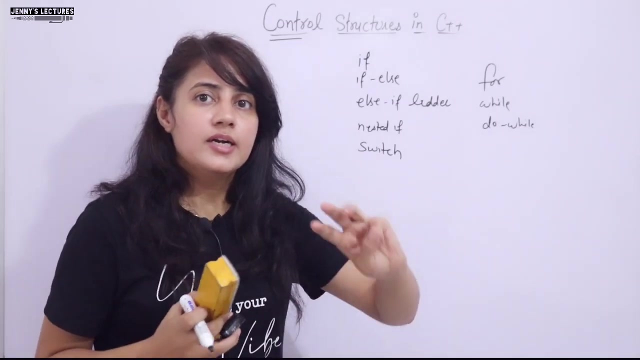 Then that would be: we do that thing with help of iterative statements, and iterative statements are for loop while loop do while loop loops. Simply you can say loops, those comes under iterative statements or iterative control structure. So basically three types of control statements: sequential, that is by default. 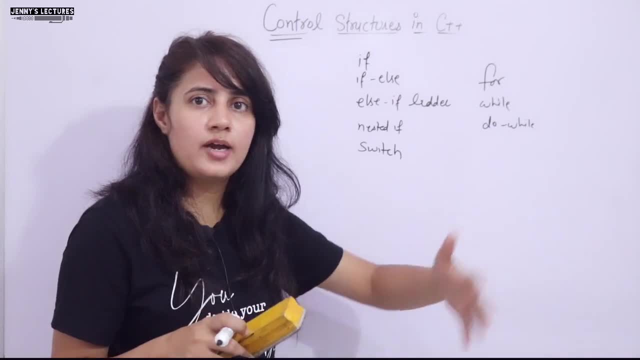 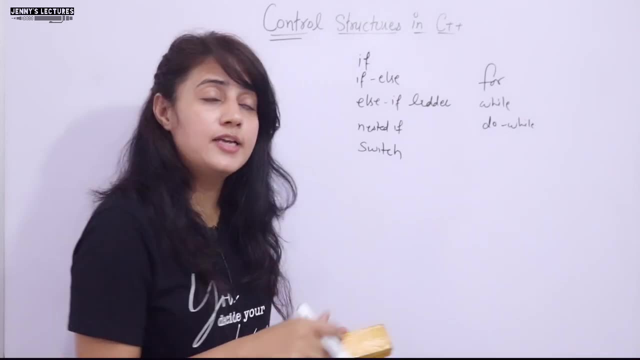 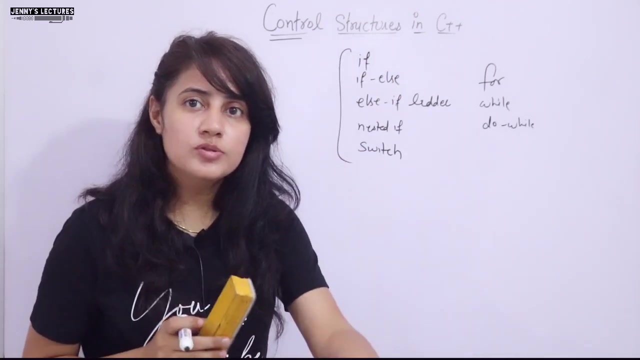 till now, whatever program we have run, I think that is based on that sequential execution of the statements right. Second one is selection that we will execute, that we will implement in a program with the help of these statements right. Next is iterative means: loops for while and do while right. 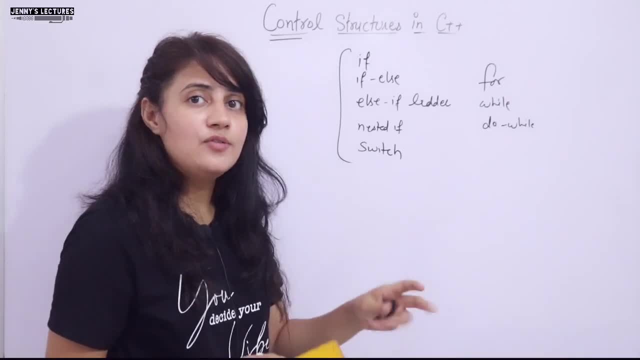 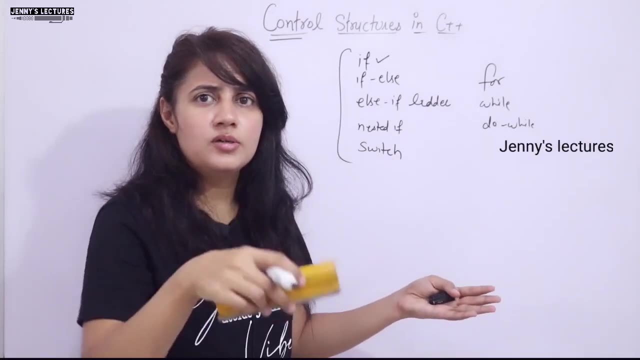 One, while we will discuss everything. So in this video, basically, we will discuss about if statement. it's not like that. if is simple, right, If write down some condition and then some statement. no, we can do some tricky things with this. 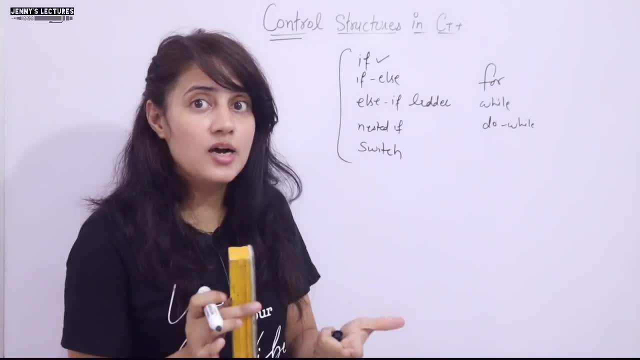 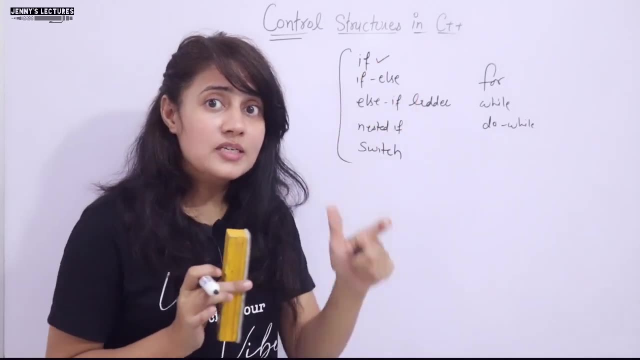 If now, whatever things, whatever tricky questions can be asked based on this if simple, if maybe it seems like it is simple one just skip the video. but we'll be discussing some tricky questions with the help of this if statement that generally they ask in competitive. 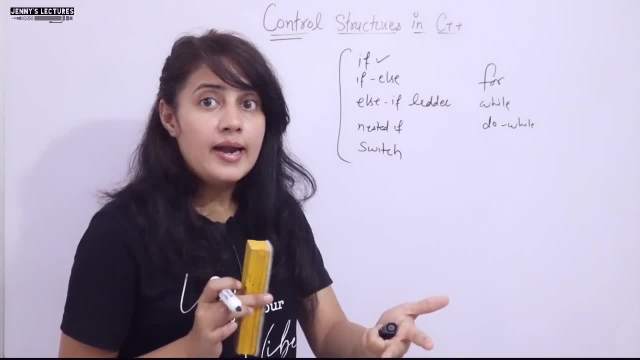 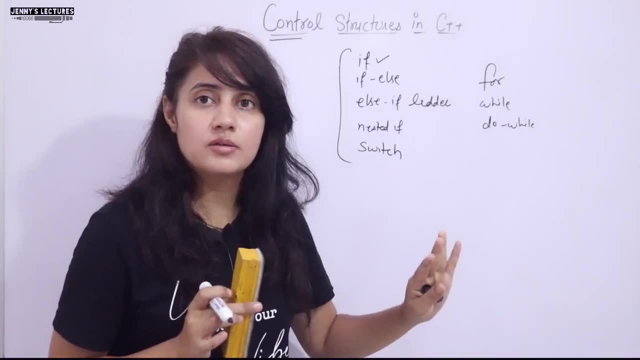 exams or interview or viva, and at that time will be shocked like I haven't tried this thing with if. is it really possible with if, Or definitely you will give wrong answer. So those things, those questions, those tricky things we'll be discussing in this video. 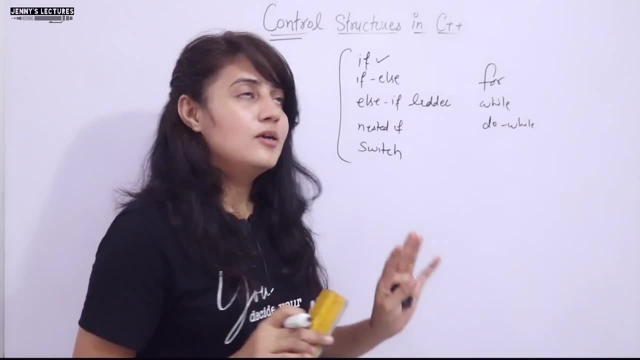 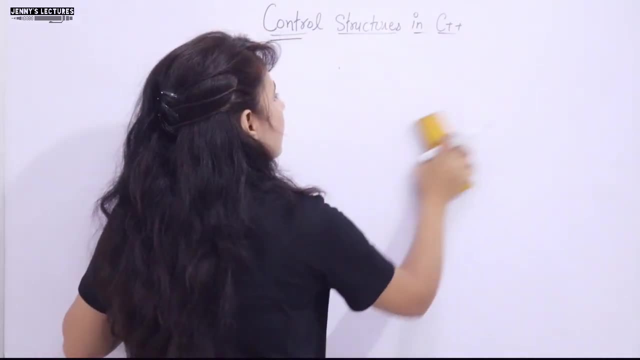 So this video is going to be really important for you guys, right? So in this video, simply, we will discuss if statement, if decision making statement, right, With the help of some programs, or you can say some examples, three or four examples. 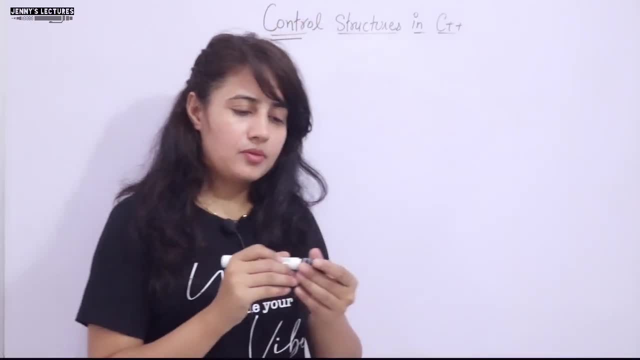 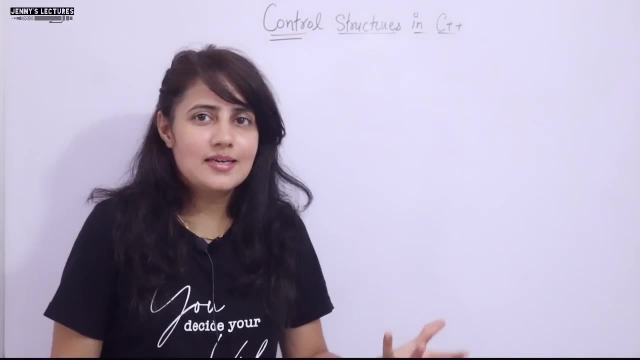 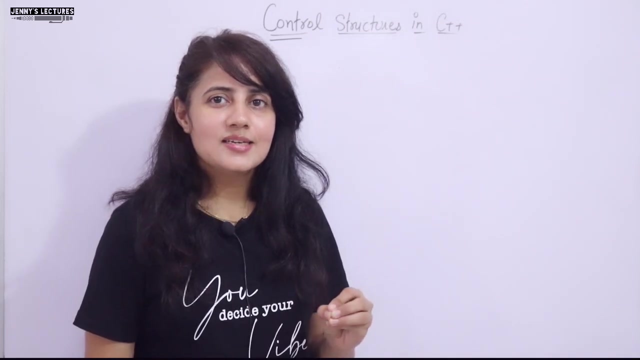 right Now. see, let's take one example. You want to go for a coffee, Maybe with your girlfriend or boyfriend. let's take a simple example. right, You want to go for a coffee. So the condition is, obviously, you will see how much money you have saving, right? 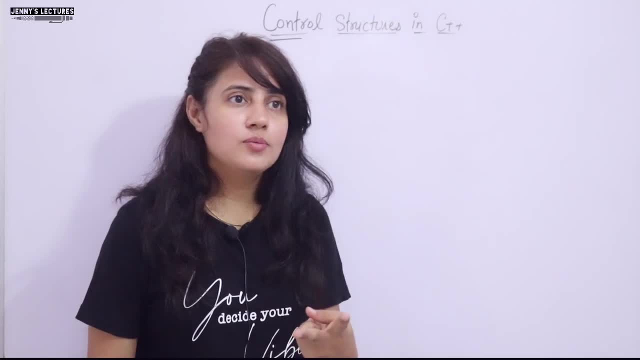 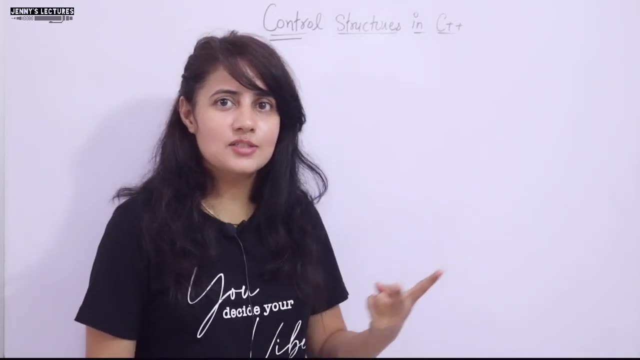 So if you have, you are two people. So if you have more than thousand rupees, you can go in Starbucks. coffee in Starbucks. Obviously that is expensive. Maybe with coffee You can go in Starbucks. You can take some more item also. 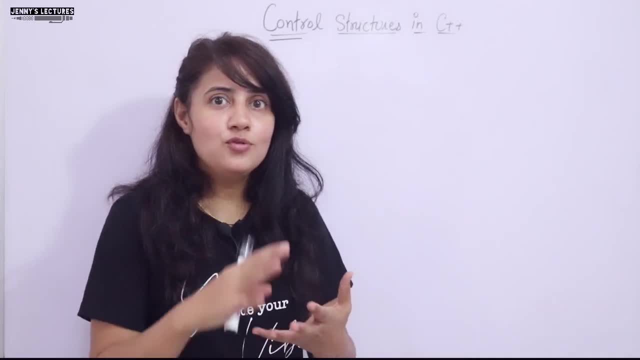 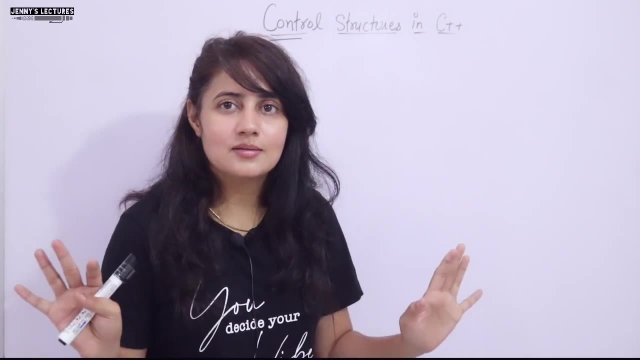 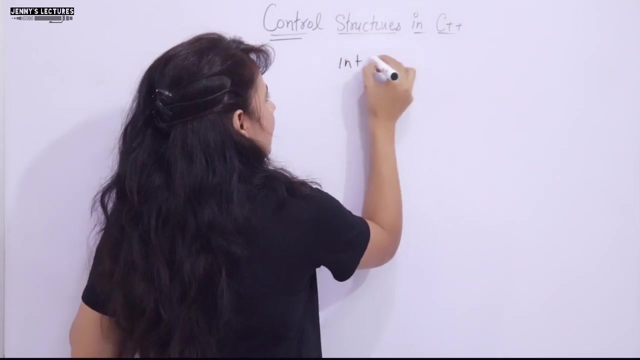 So at least you should have a hundred rupees. You will see your budget. If you don't have thousand rupees, then simply what you say: let's go home. That's it right. So how you can implement this thing, like I'm taking in mail, I'm just writing: 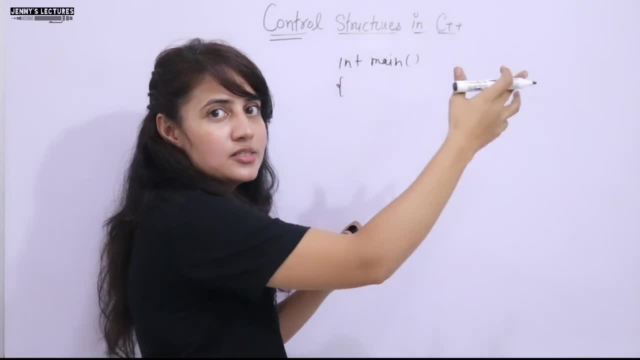 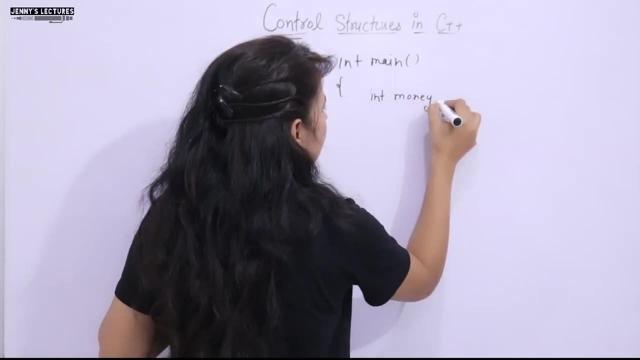 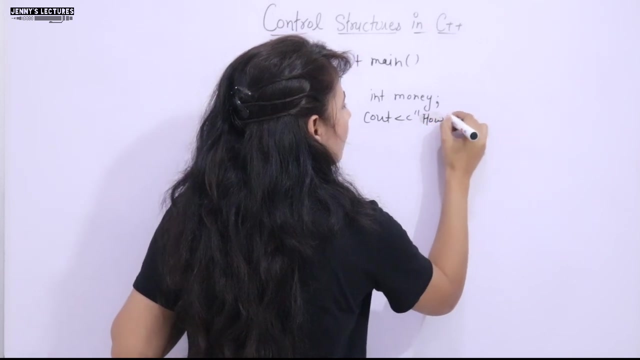 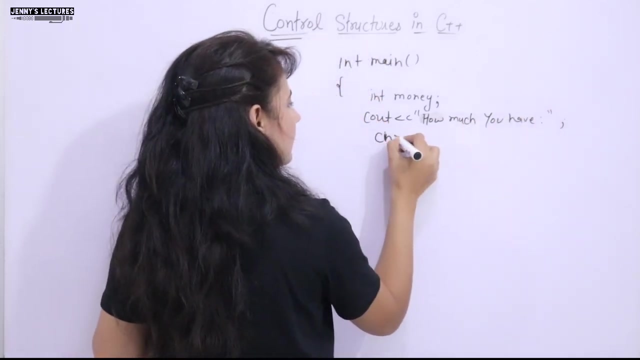 I hope you can write down these header file. hash include IO stream using namespace STD. These two things by default, right, Okay, Now int money. then simply we will enter, or you can say how much you have. right, Then cin. this is what input output. how to take input using cin. how to print output. 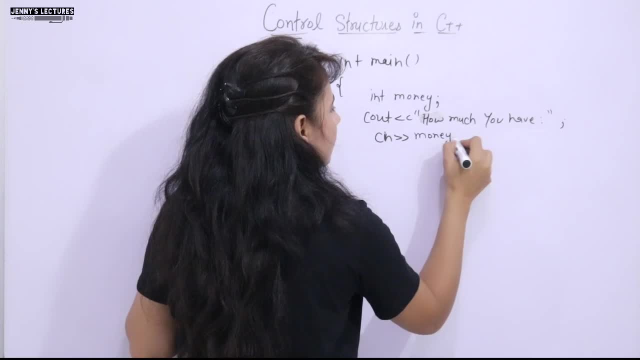 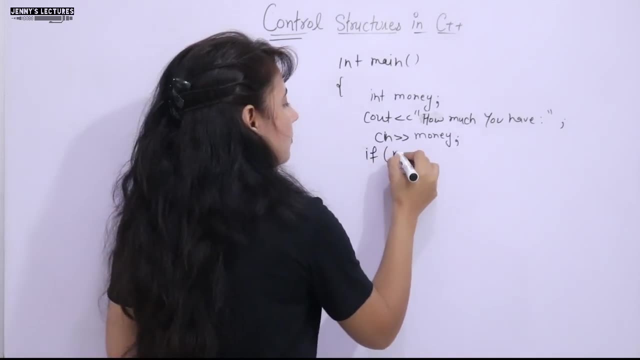 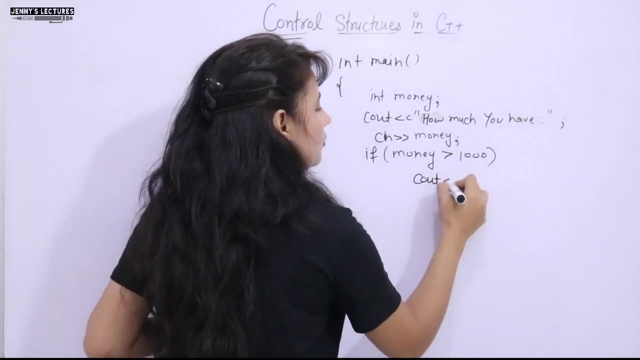 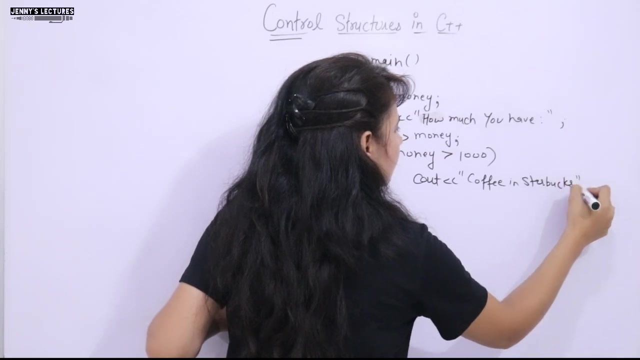 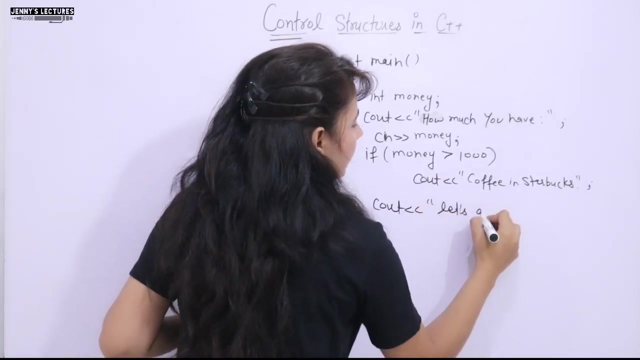 using cout, right Then money. Now we'll check condition: You check your pocket, How much money, How much money you have. If money greater than thousand, then simply cout. I'm simply printing coffee in Starbucks. After that I'm printing cout. let's go home and return the money. 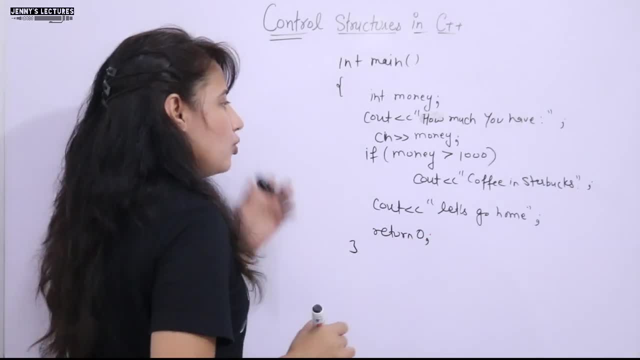 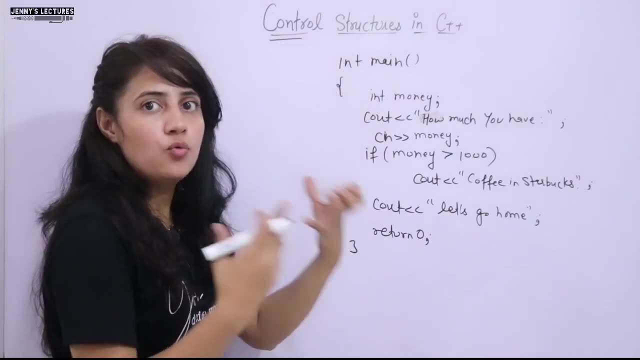 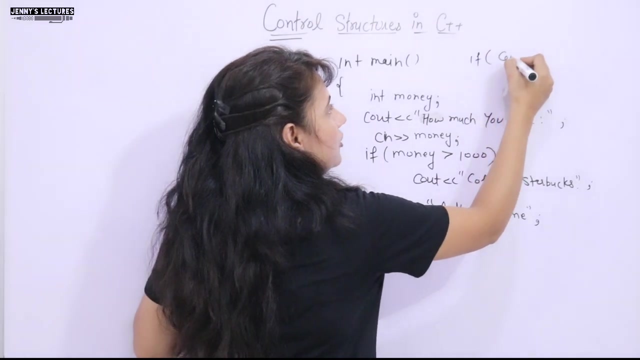 Okay, Return, zero right. So first of all, before explaining this, let me just explain this. you know general flow chart of general working of if statement right. The general syntax is simply: you will write if, then some condition, and then here you. 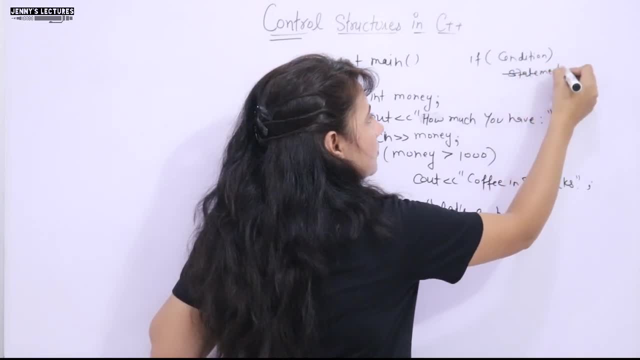 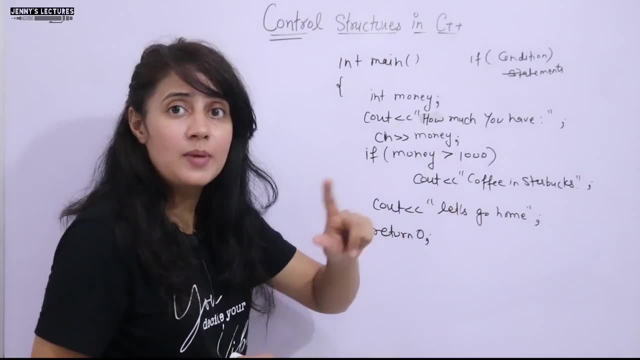 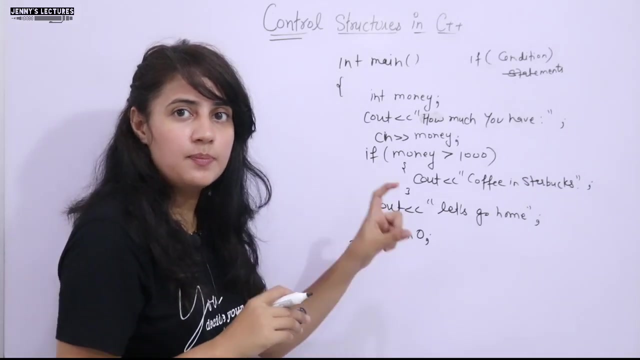 will write statements. You can write single statements. you can write multiple statements. if you write single statement, simply you can write this thing. If you are going to write multiple statements, like two statements, then you have to put this curly braces: multiple statements you can. you have to put these curly braces. this is. 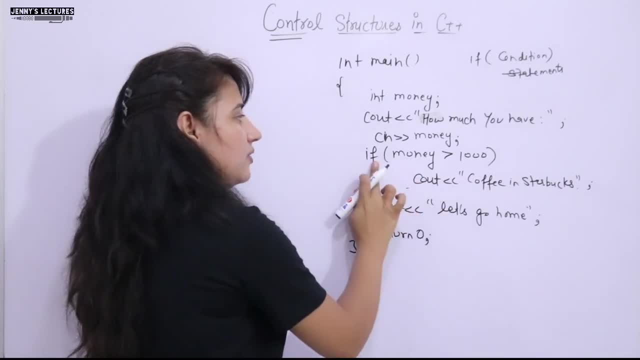 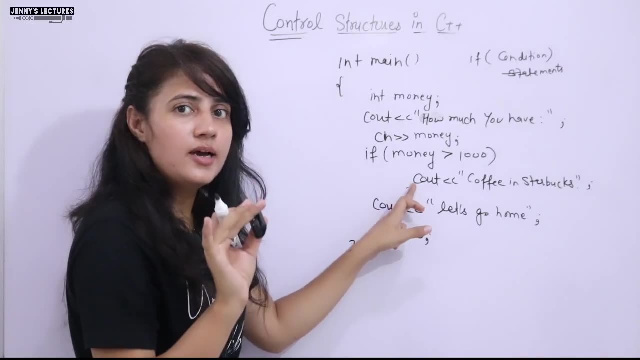 what you can say: block of statements. If single statement you are writing in this if block, no need to put this curly bracket right By default. this one statement only would be considered as a part of if block right. This statement would be after if statement. you can say: 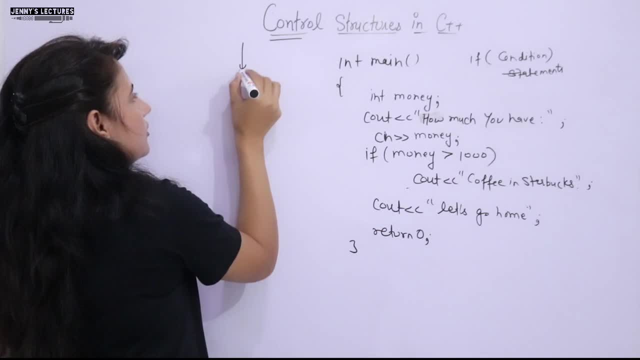 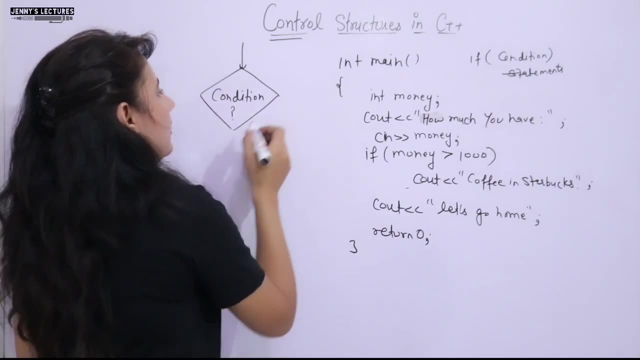 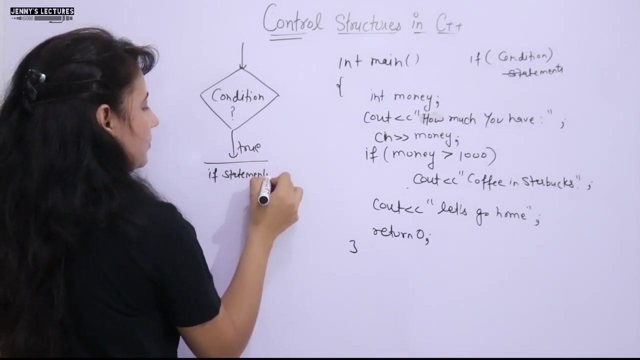 Okay, So general flow chart can be something like this: This is just, you can say the entry, then we have some condition if condition- right. If condition is true, then we have if statements, If you can say if block statement- right. 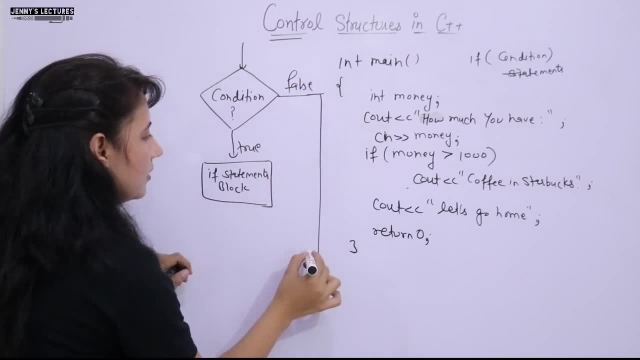 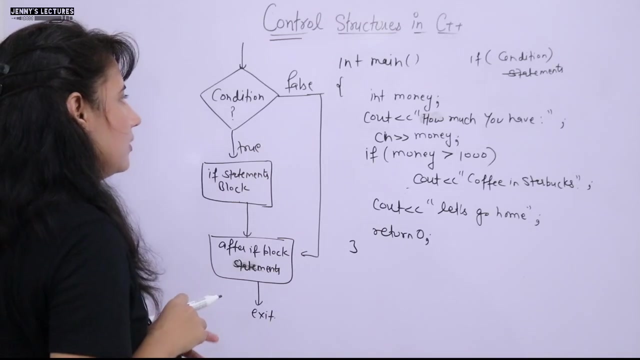 If condition is false, then simply condition is false, then whatever. after this, if block, whatever statements are there, those would be executed So that you can say after: if block statement right Now, this, and after that you can say exit. 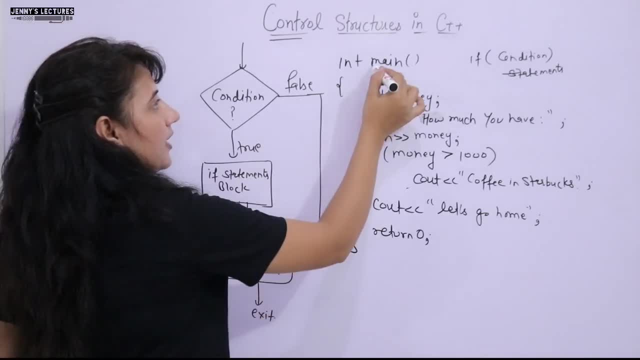 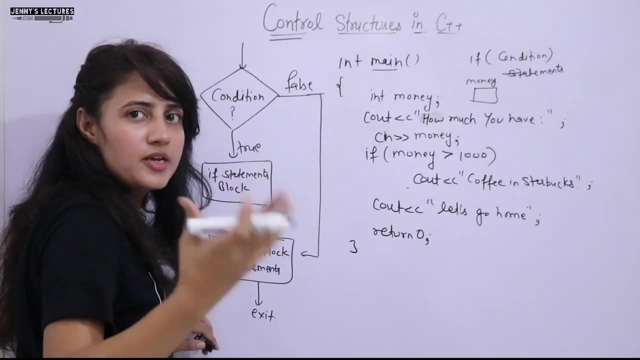 So in this case, let's see, this is the flow chart, This is the entry main, Then money. That money variable would be located, located some space in the memory, 4 bytes right. Then see out. it would be printed on the output screen how much you have. 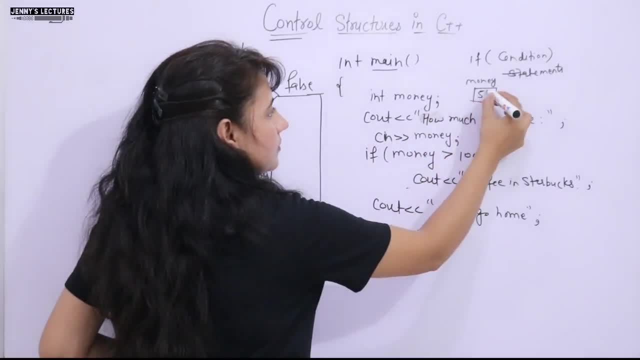 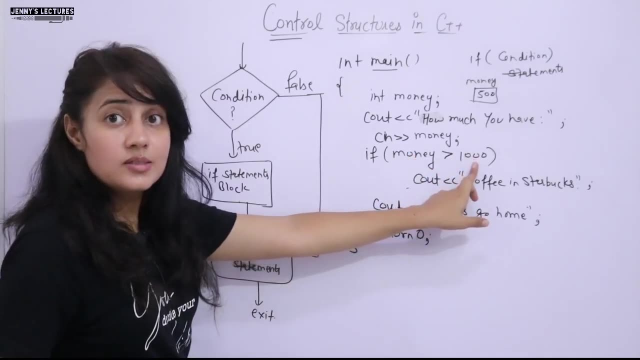 Then see in money. suppose you have 500 rupees. 500 would be there Now. check the condition: money greater than 1000, is this true? No, you have 500 rupees. money is less than 1000.. 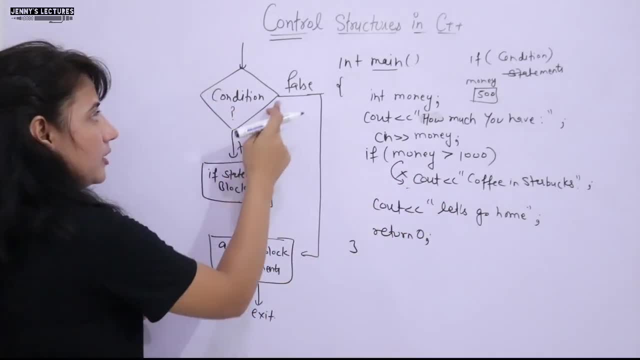 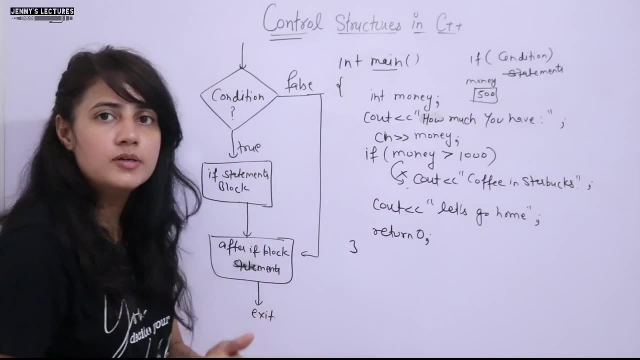 So will not enter into this. if block: Okay, Because the condition is false. then after: if block condition. after if block: this is the statement. See out, let's go home. So this would be printed: Let's go home. 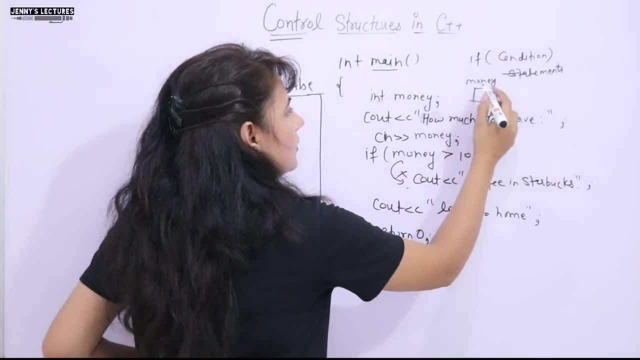 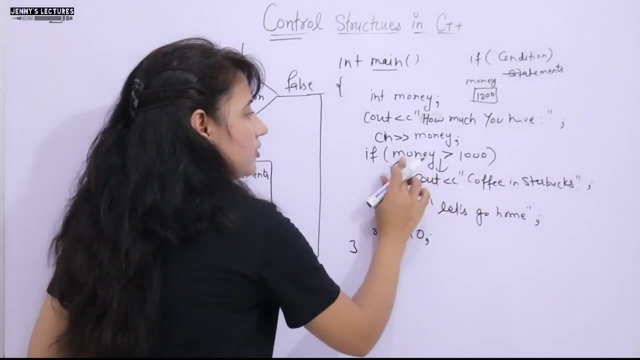 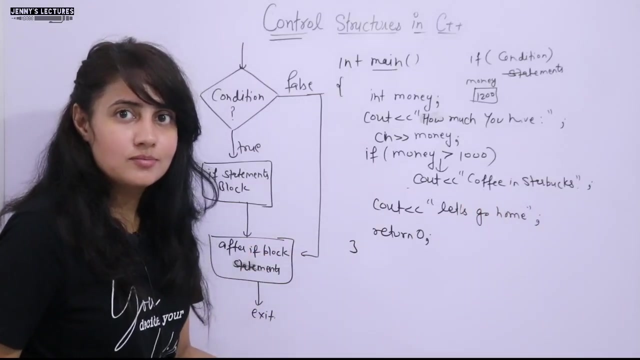 Right, If you have, you are entering money. suppose 1200 rupees you have. so the condition is what? True now. So we'll enter into this if block, and what would be printed? Coffee in Starbucks, Now you can take. coffee in Starbucks, you can have. 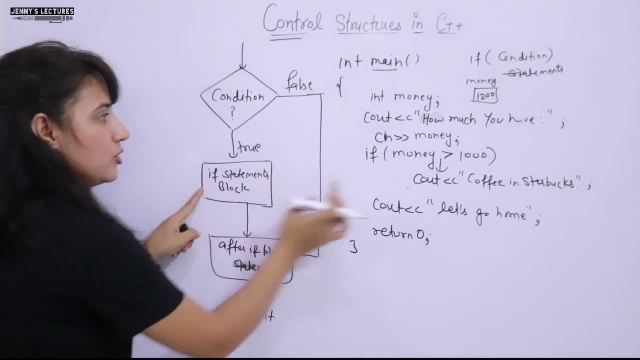 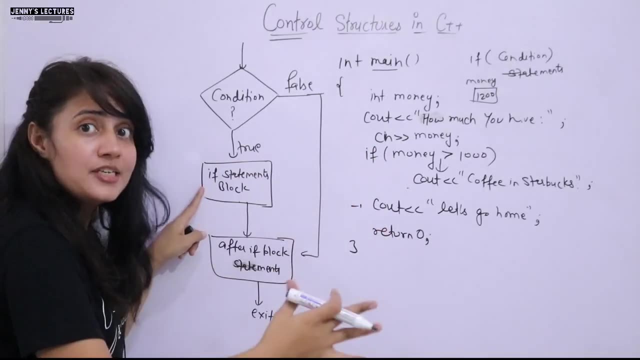 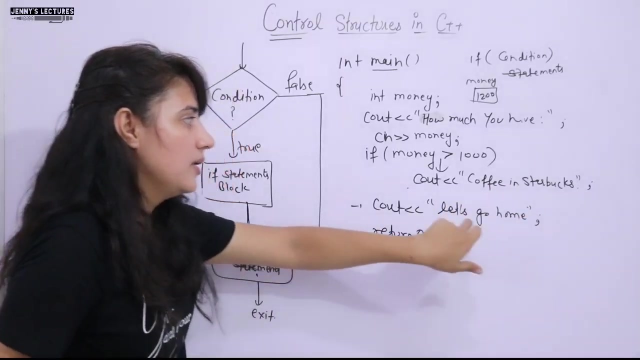 Right, If true. If true, then if statement block would be executed means this would be printed: coffee in Starbucks. After executing this, whatever is written after if block, that would also be executed. This is the flow. Then, after if block, Now in this case output, output would be coffee in Starbucks. 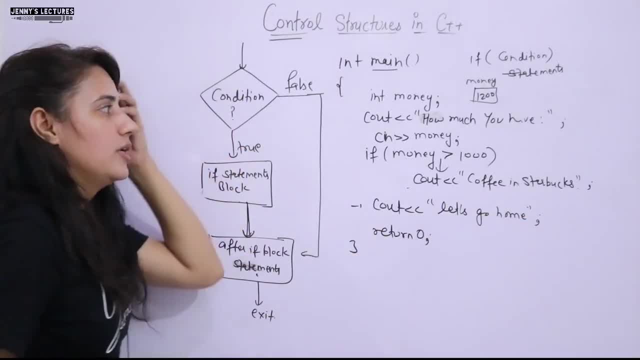 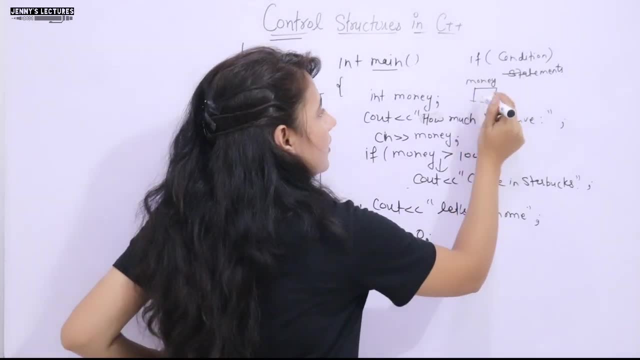 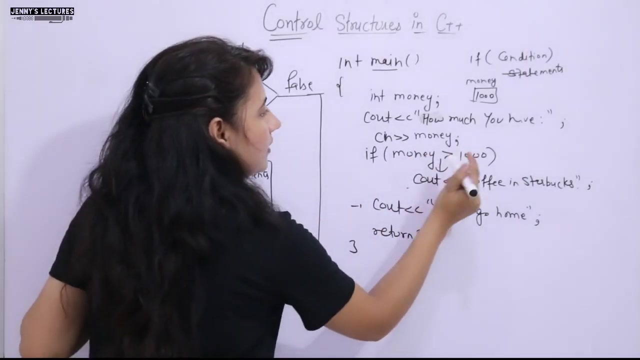 Let's go home. These two statements would be printed on the screen right. So this is the working of the simple if block Now up. I'm just writing 100,, sorry, 1000.. So if you want to, you know, change the condition like: money is greater than and equal to 1000,. 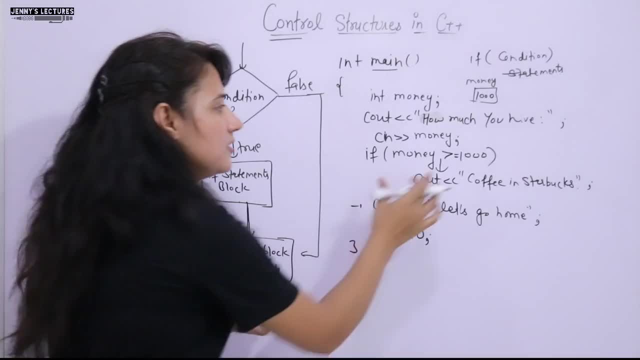 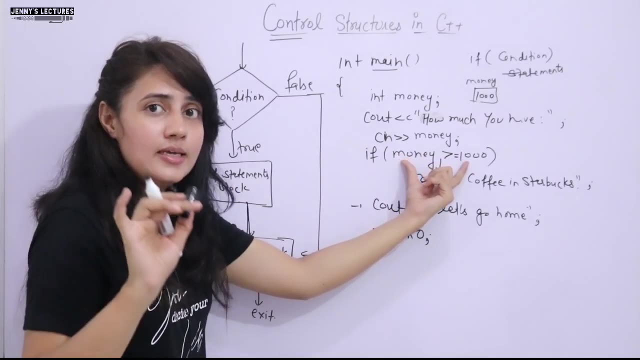 then also you can have coffee. So this also you can take. This is the condition. This condition can be any expression or any constant value, but this should be evaluated, at last, finally, in a Boolean value. either true or false, That's it. 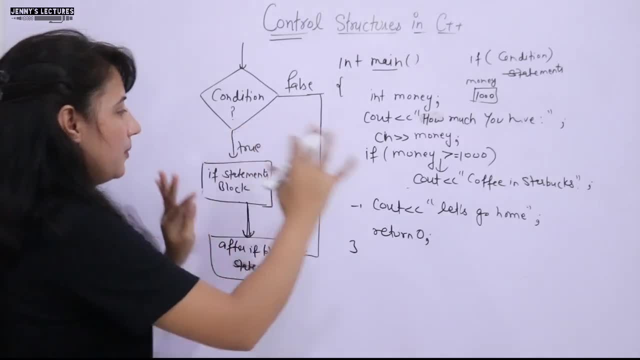 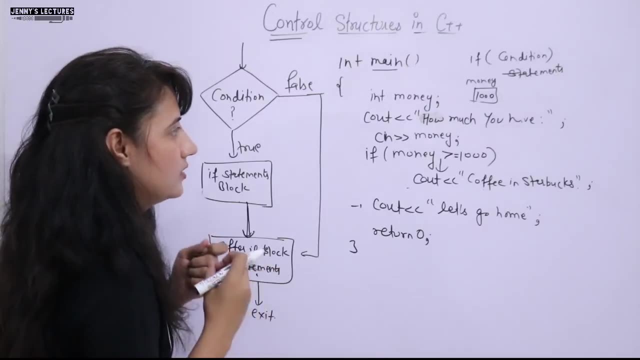 Right Now. Okay, I hope the simple working is: You have understood the simple working of coffee. You have understood the simple working of this if block, Now let's do some tricky things with this. if Sometimes, if I put like semicolon here, 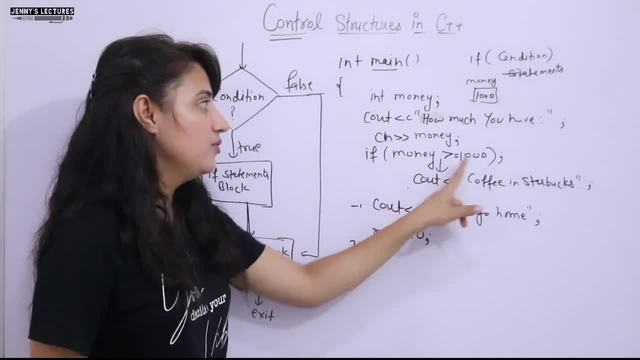 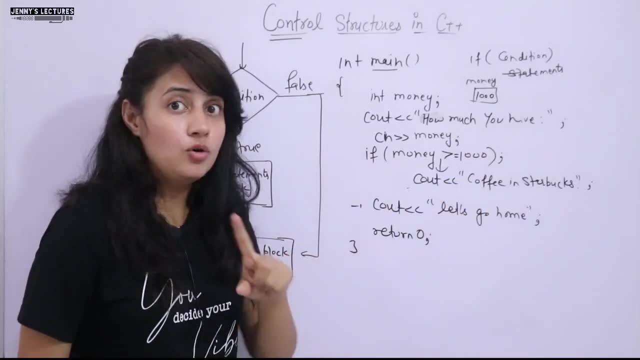 Now maybe you think sometimes they ask this type of questions after: if they put semicolon. Now maybe you will think this is an error, because we cannot put semicolon after this. if You will say it is an error, No, it will not give any error. 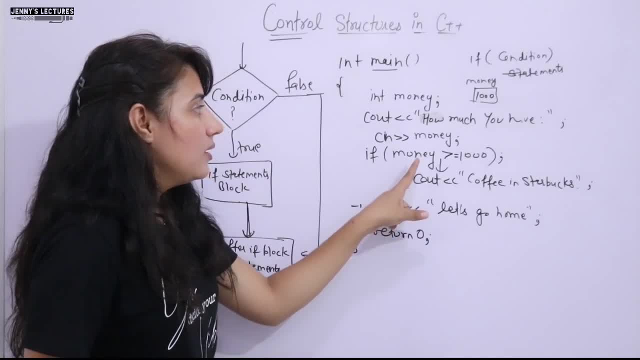 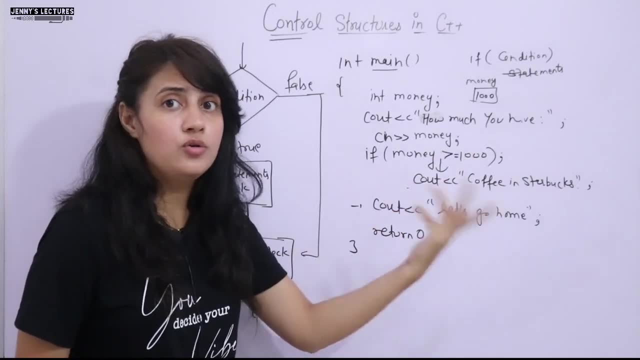 Simply program would run, Then what output you will get. See, This is what you can say. This is the condition of this. if block means there is no use of checking the condition now You have. you have just terminated this if condition here. 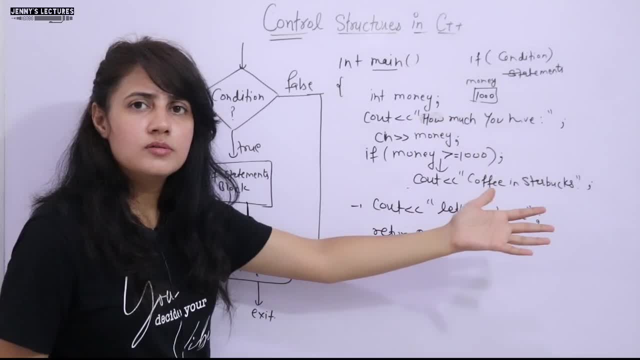 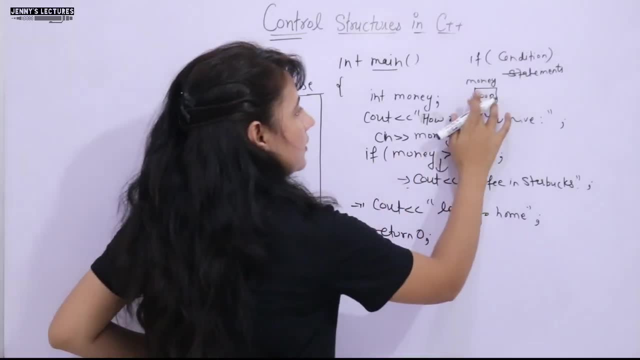 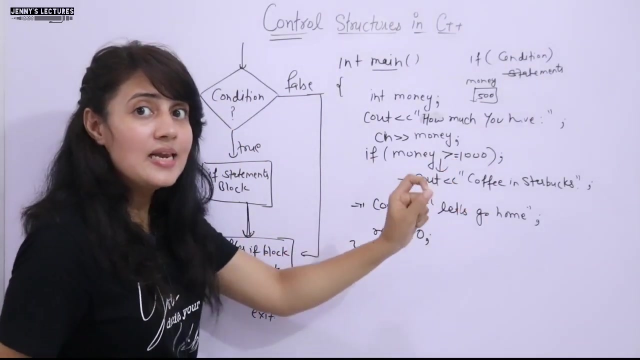 So in this case, whether the condition is true or false, this would be executed. the if block as well as the after if block would be executed. So if I'm here, just I'm writing, I have 500 rupees. Maybe you think that the condition is not true, but still, because you are terminating, 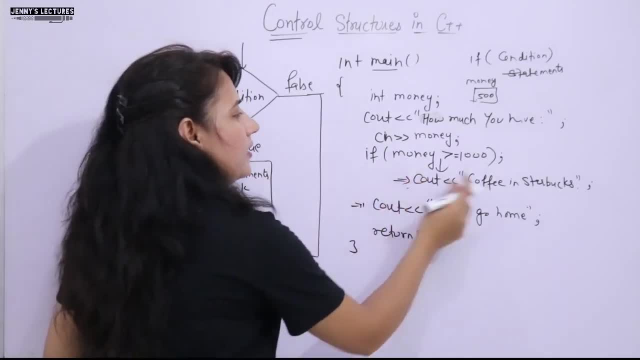 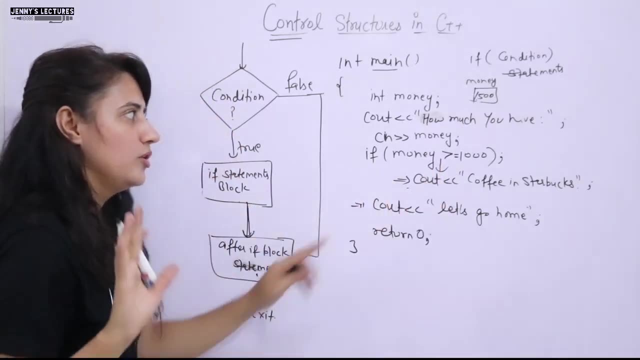 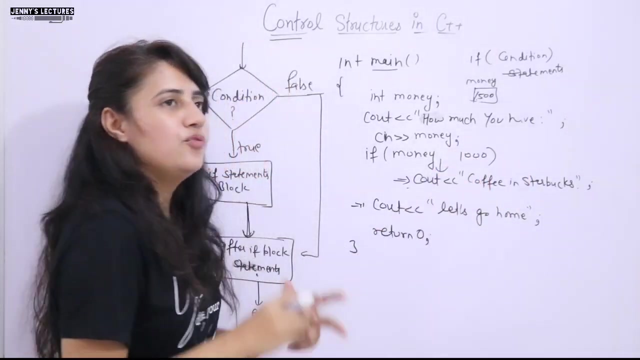 here. So use of checking the condition. still it will print coffee in Starbucks, Let's go home. If I write 1500 rupees, still it will print coffee in Starbucks, Let's go home. So it is just terminating of this, if block, right, if I want to check equality condition. 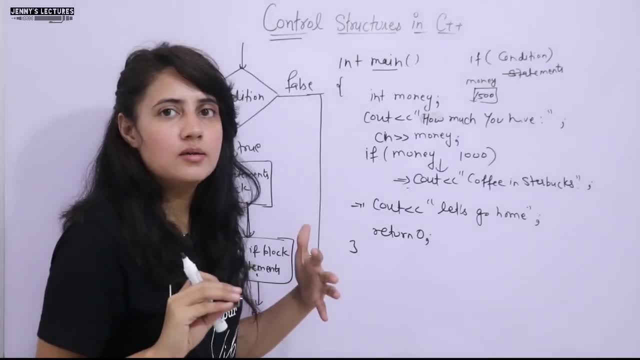 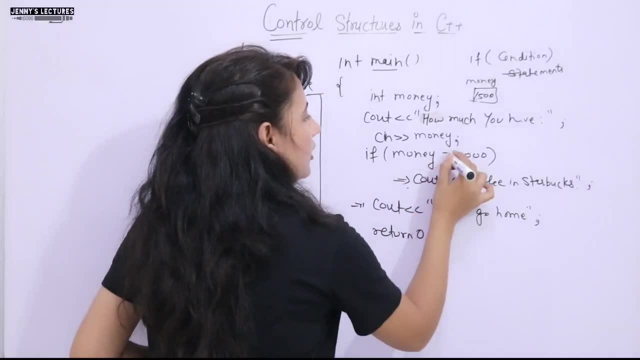 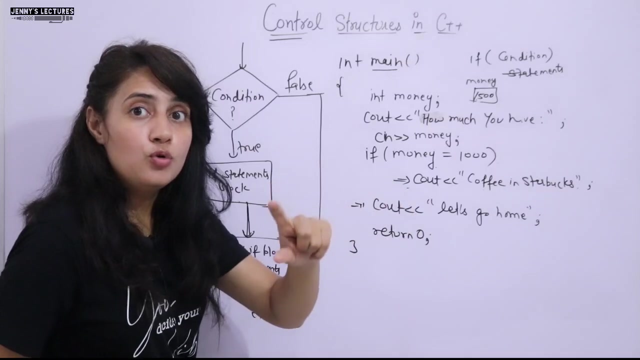 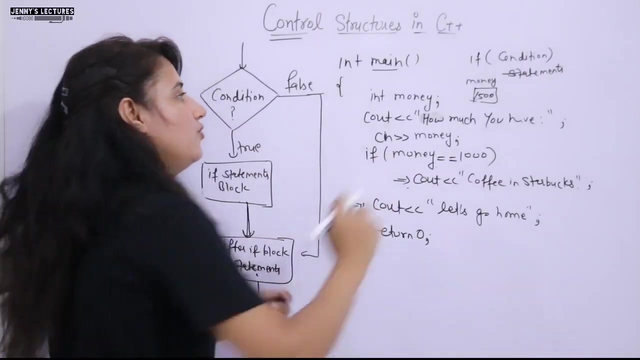 if money is equal to thousand, then only we will have coffee in Starbucks means money is equal to right. So sometimes maybe you write money equal to thousand rupees. No, In programming language this is what assignment operator. If you want to check the equality, the equality operator is double equal to now. it is fine. 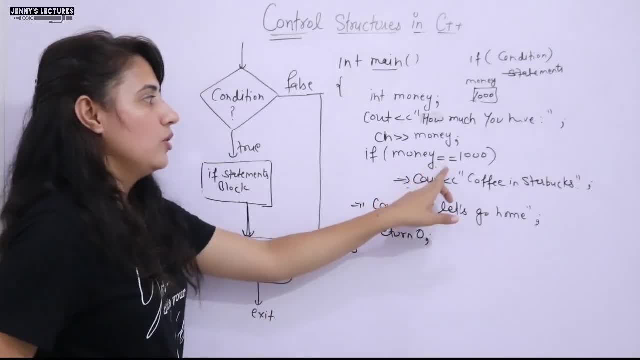 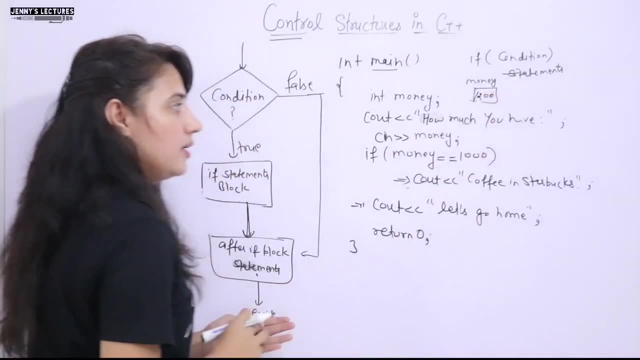 If money is now thousand, money is equal to is equal to thousand. obviously, condition is: to enter into this coffee in Starbucks, Let's go home. If money is 1200, money equal to equal to thousand. no condition is not true. So not enter into this block, simply print. 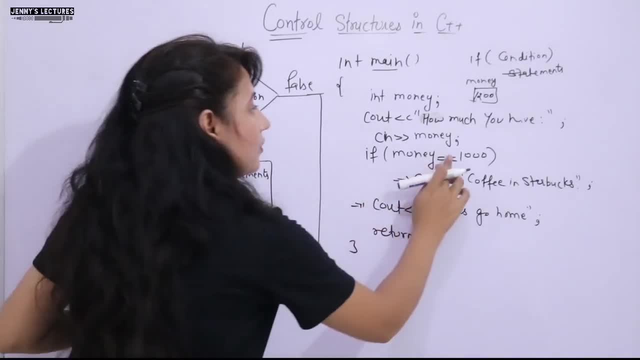 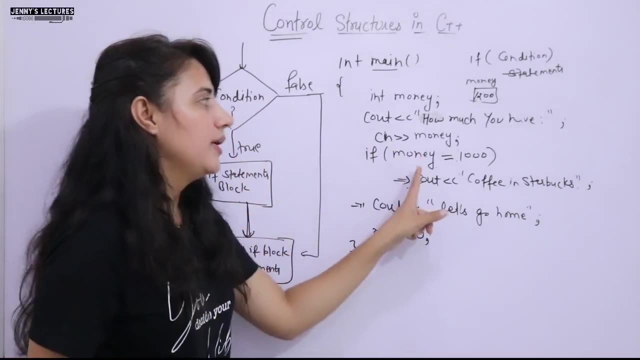 Let's go home, Right. If you write this thing, money equal to thousand. sometimes they ask this type of question also. So it is what? simply assignment operator, Suppose money. I'm entering 12000 means you are, means you know. you will think that this. 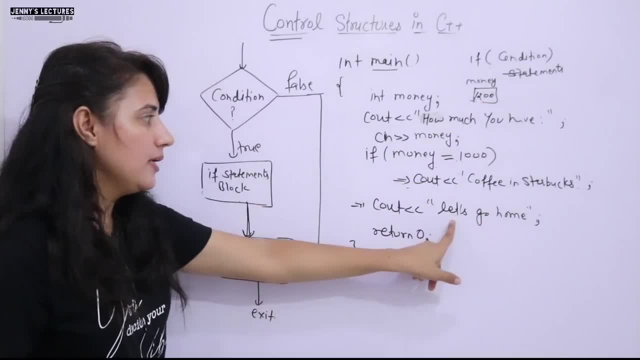 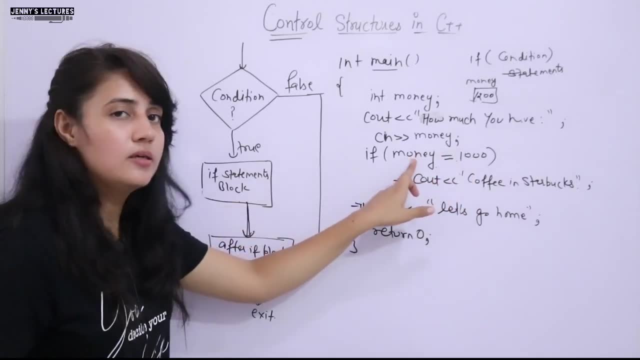 condition is not true because money is 12000.. So simply print: let's go home. No, It is not equality check condition. Simply it will assign thousand to this money. Assignment operator is assigned right hand side value to level Let's go home. 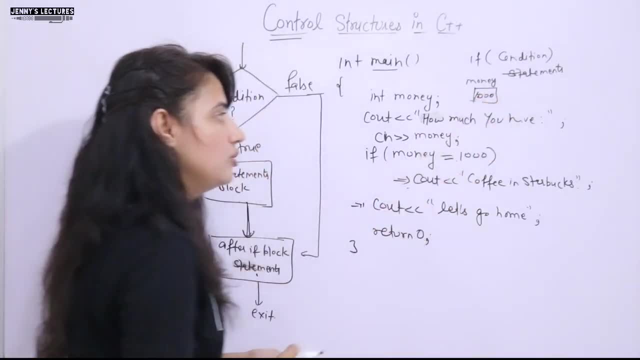 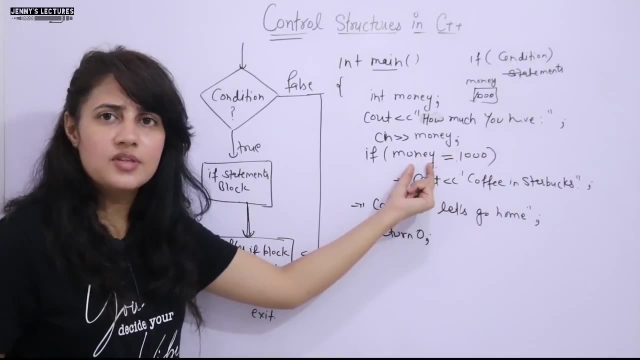 Let's go home. left hand side. So now the money becomes here thousand. So this is what money is: thousand, So simply other than zero. whatever you write, whatever is there in this, within this bracket of this, if that would be considered as true. So this is true. 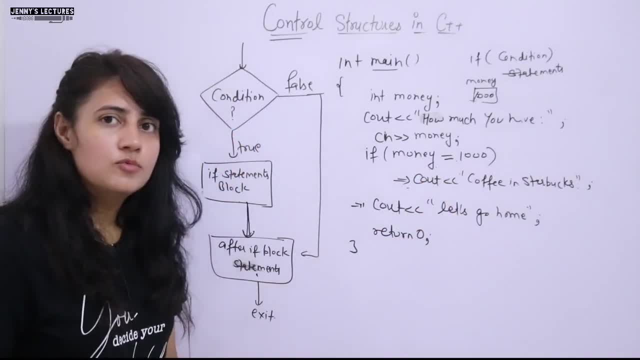 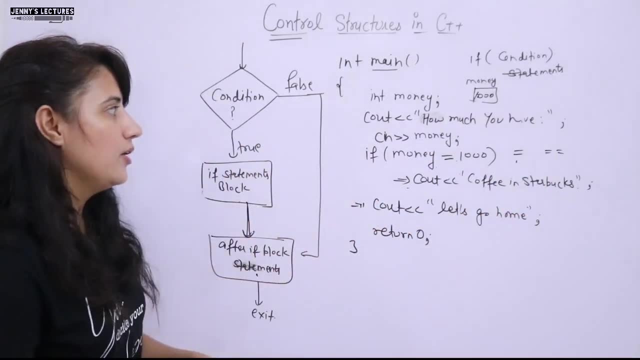 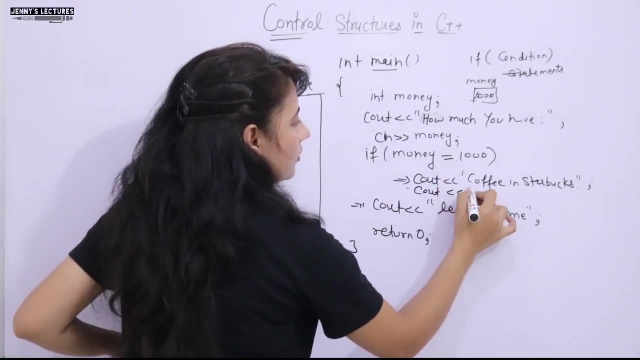 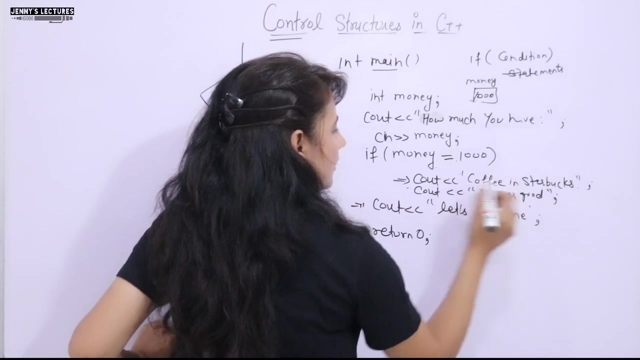 It will print coffee in Starbucks. Let's go home. So please be careful while you use equal to and double equal to. this is assignment operator. This is equality check Right. I hope you got this thing Now If I want to print here in if block: see out coffee in Starbucks, and it was good. 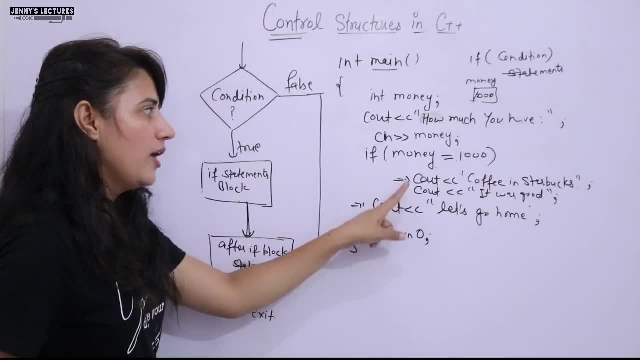 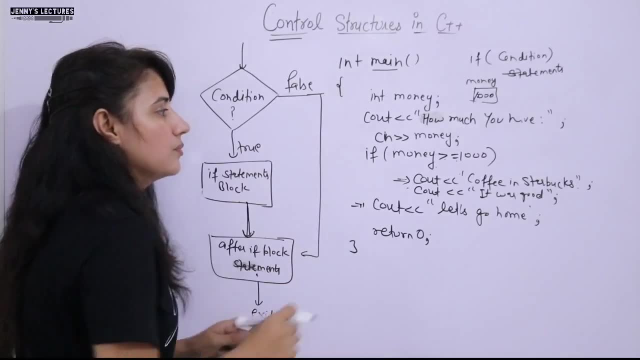 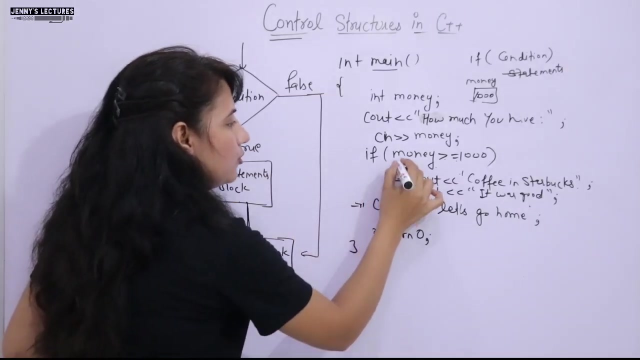 These two lines. I want that these two lines should be a part of this. if block money is greater than equal to thousand. So if you don't put these curly bracket, then what will happen? I'm not putting Suppose, I'm putting curly bracket. 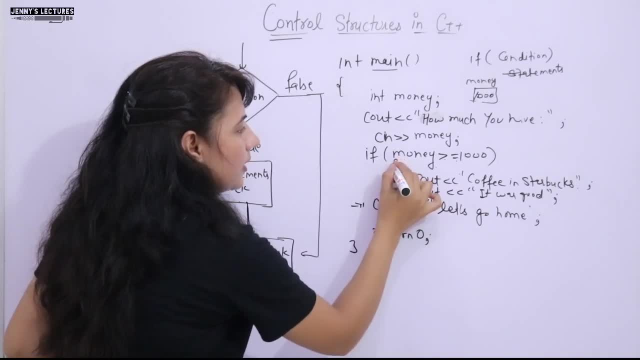 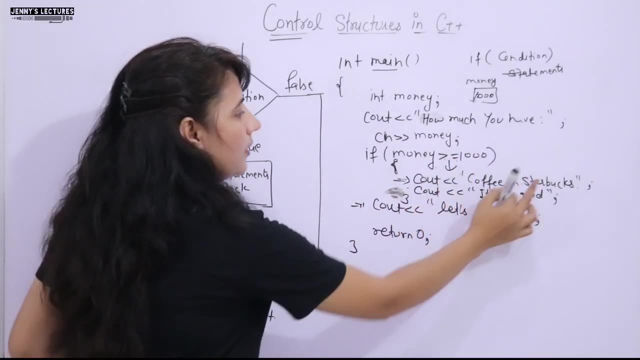 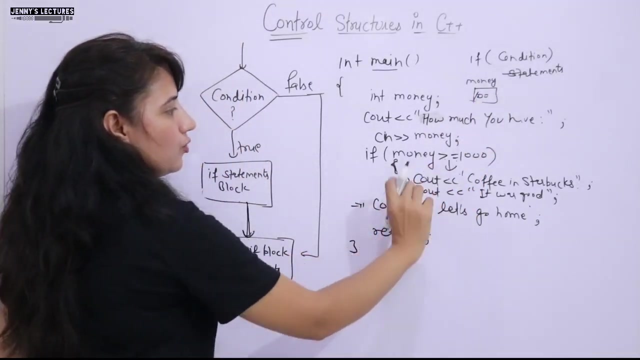 Suppose I'm putting curly bracket first, These two lines in these curly brackets. So now money is thousand condition to you. will enter into this. if block what would be printed coffee in Starbucks- It was good, Let's go home, Right? If I have hundred rupees, the condition is not true, will not enter this control will. 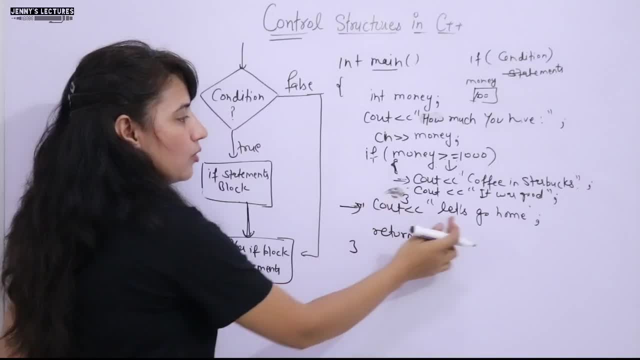 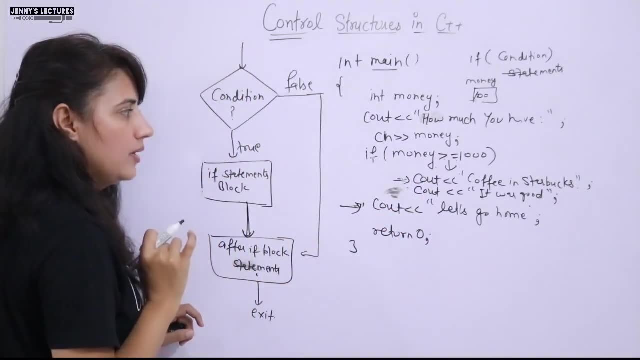 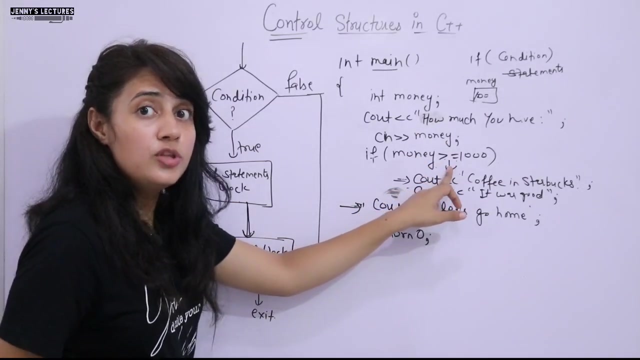 not enter into this. if block, and what would be printed? whatever is there after. if block, let's go home- would be printed only Right. If you don't put this, These brackets Right Now, what would happen if hundred money is hundred? condition is not true means you think. 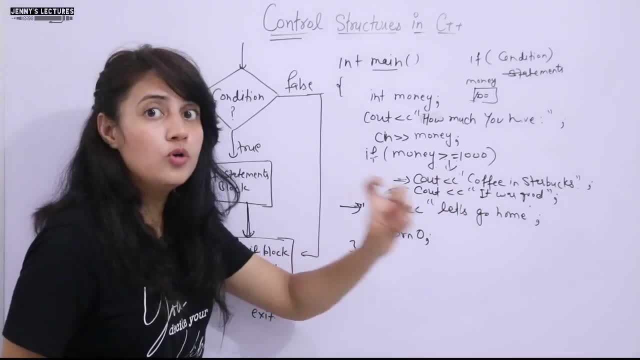 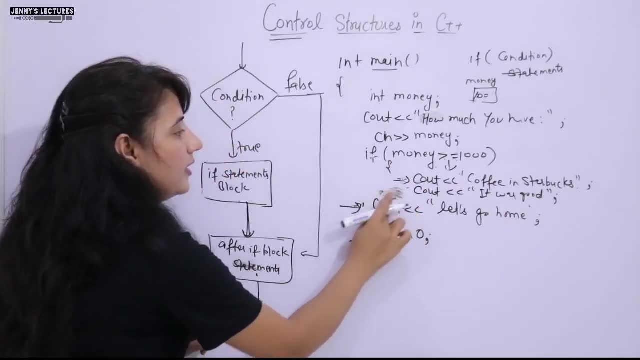 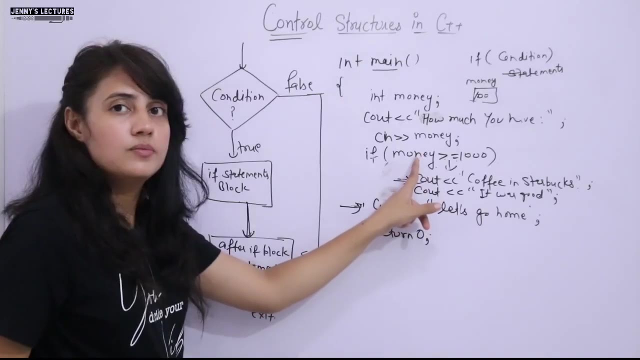 that output. output will be. will be: let's go home, but no, what would be the output? it was good, Let's go home. Why so? because you're not putting any curly bracket here, So by default, only after this, if only one statement would be considered as a part of this, if block. 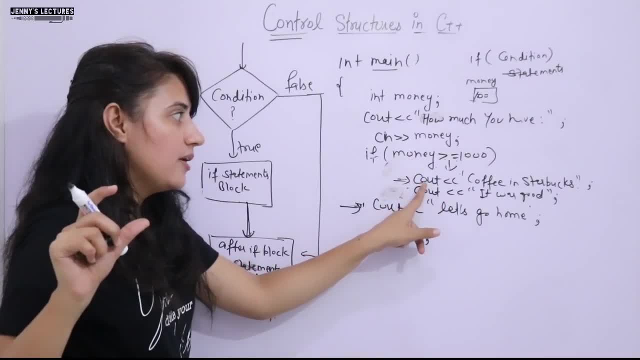 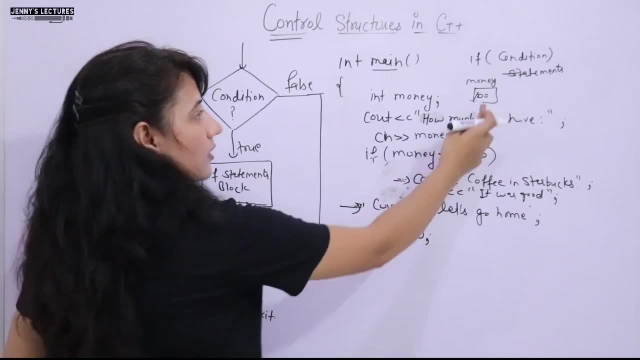 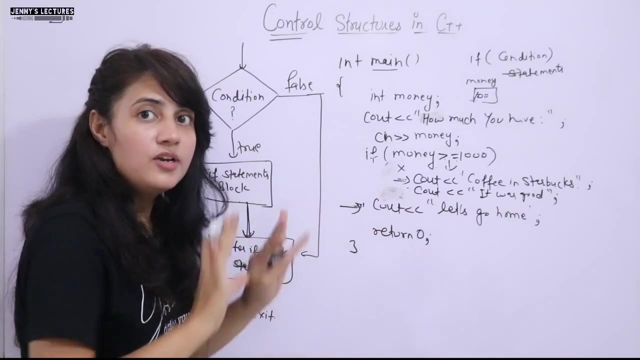 only one statement After this one statement. whatever statements are there- one, two, three, four- that would be considered as part of after if block. That is why condition is not true control will not enter those into this. if block means coffee in Starbucks would not be printed after if block. these two would be now the part of 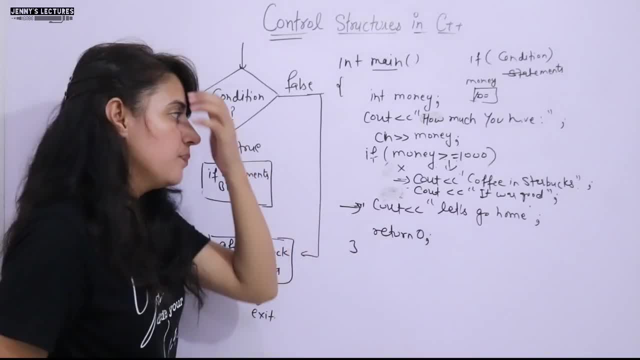 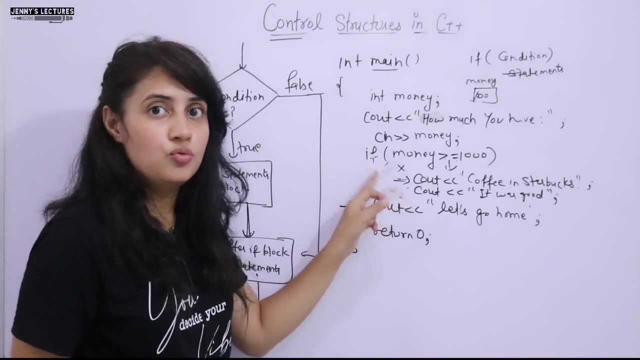 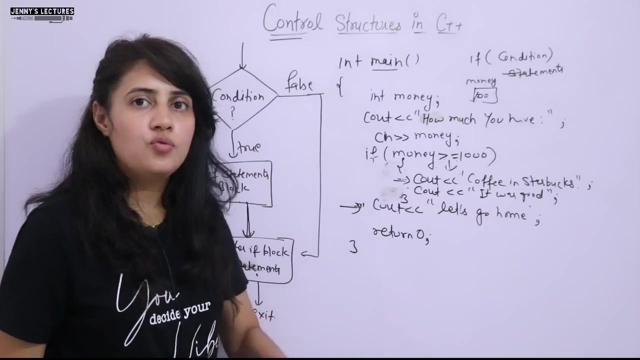 after, if it was good, let's go home, would be printed. So that's why I was saying: if in this, if block, if you want that multiple statement should be included after this condition is true, then you should put all these conditions into blocks, into these braces: one, two, three, four, five, six statements, any number of statements. you 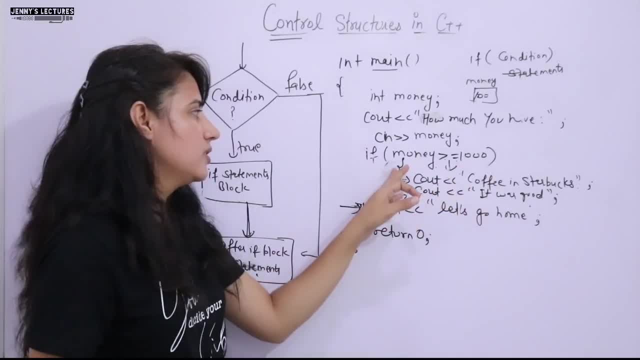 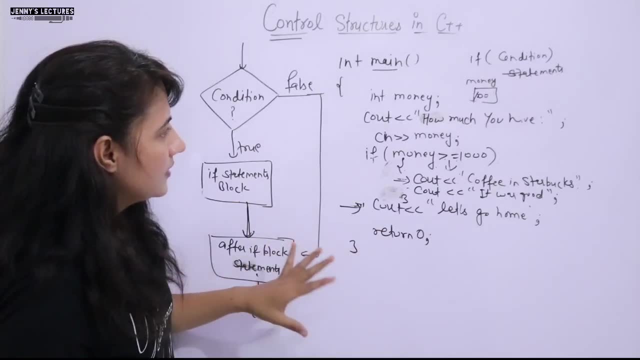 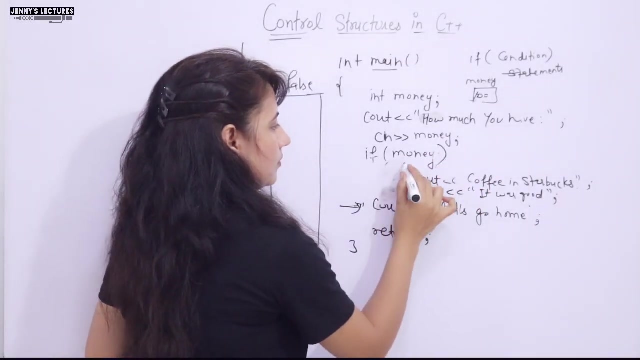 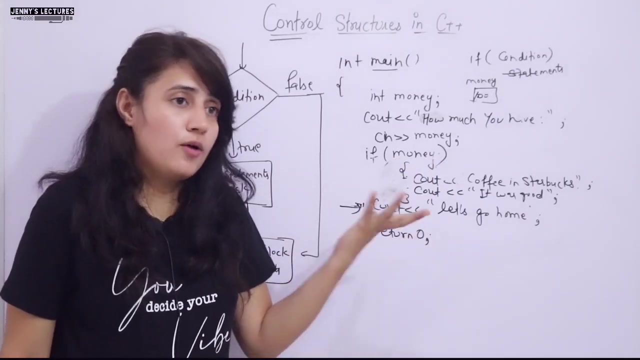 can. if only one statement is there, then you can skip these curly brackets right. I hope now everything about this if is clear to you guys and see: if simply you write money, That is also fine. it's not like that you have to put condition, that is also fine. but in 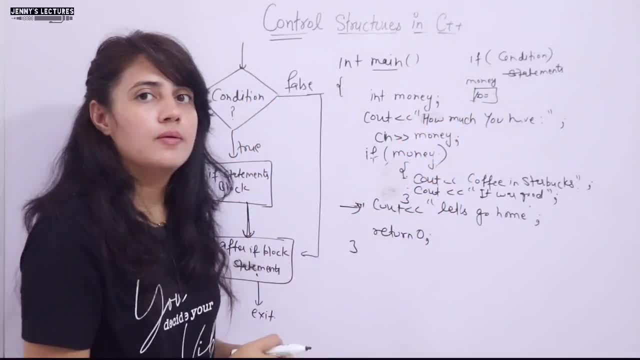 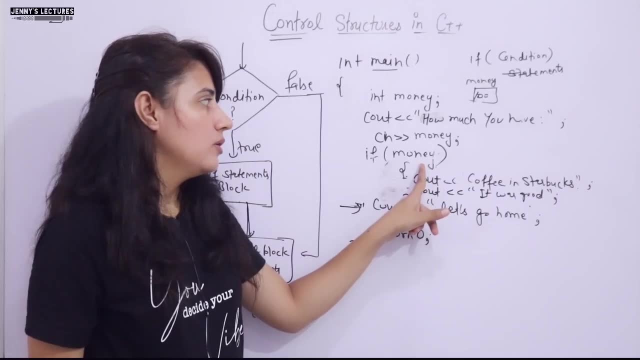 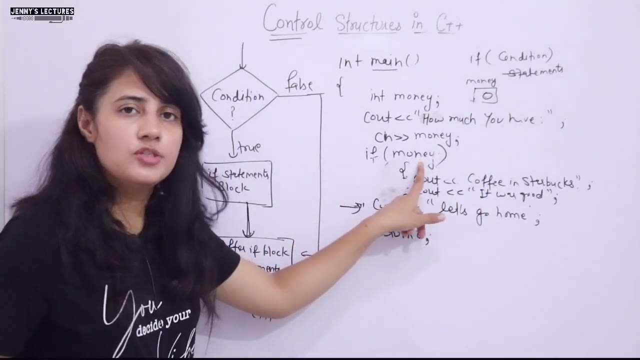 this case, if you will enter money hundred, money hundred, so other than zero, whatever is there here that would be considered as true. so this statement is true. So if block statement would be executed, then after it, if I enter money zero now, zero at this time, it is false, only right. 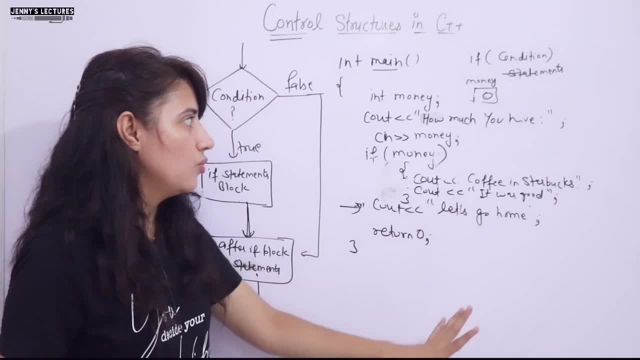 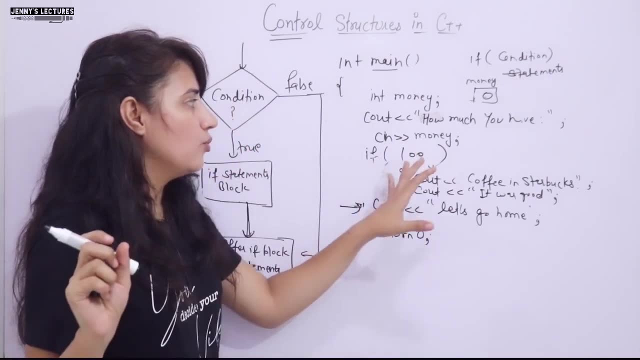 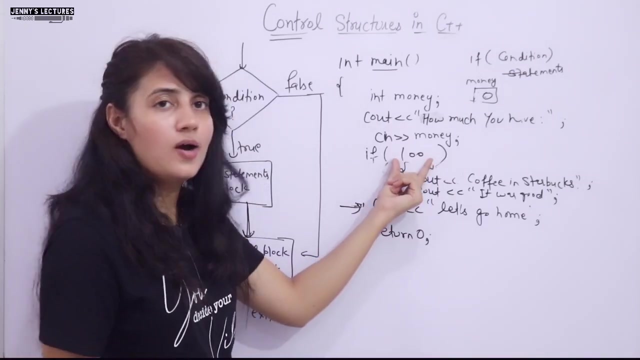 So now it will not enter into this. if block, it will simply print: let's go home. So this condition can be any constant value. if I write any constant like hundred, So always it would be true. hundred is always true. there is no chance of any, you know, false. 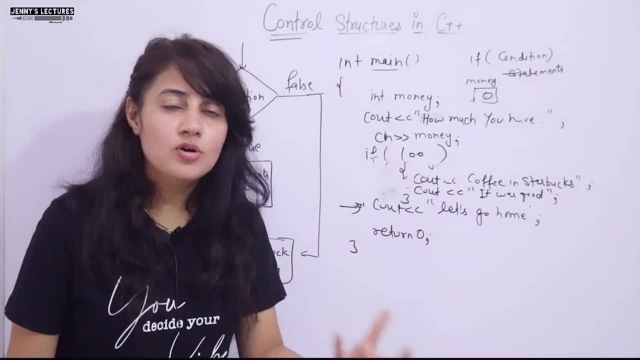 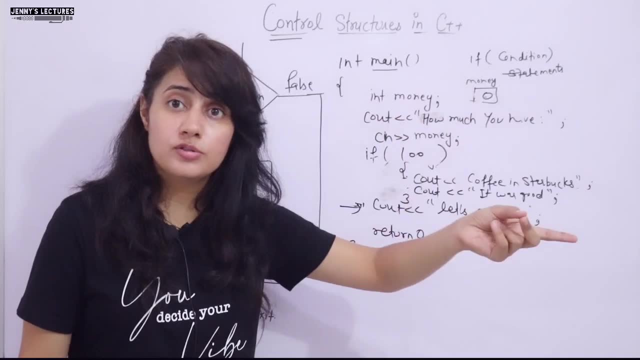 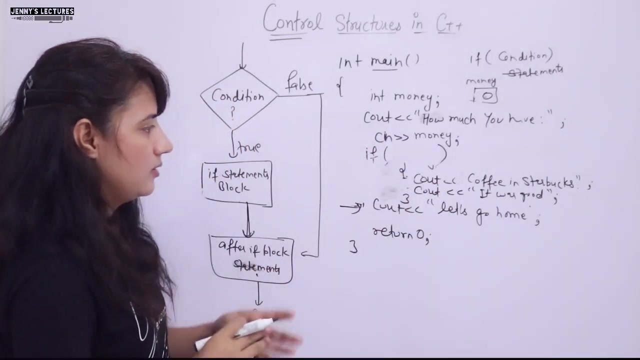 statement here or false condition here. So any constant, constant thing you can write, any expression you can write, but that should be evaluated ultimately into. if It should not seen into a Boolean value, either true or false, Then only this if will go right. I hope now the working of this if is clear to you. 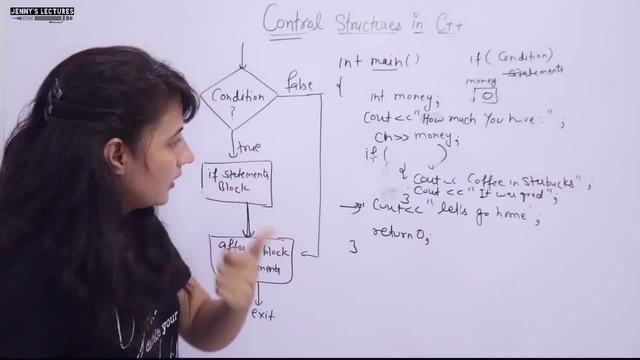 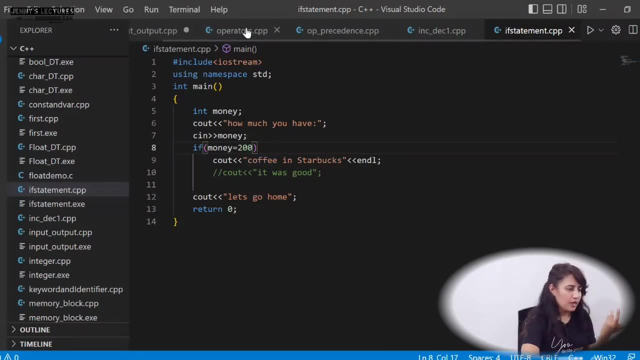 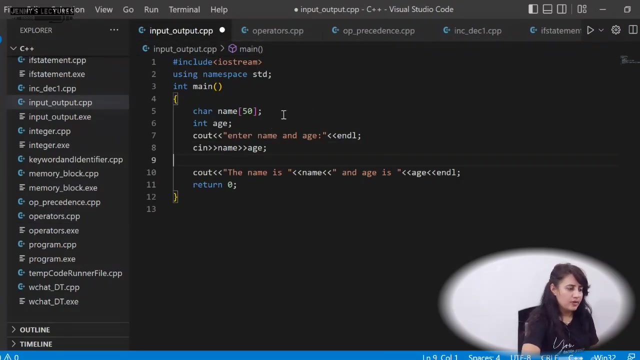 Let's, ah, see this thing with help of practical, with the help of a program. Okay, so this is that program. See, before this program, till now we have written program with, simply, they were following that sequential control structure, right? No, if else nothing, Simply, one by one, line by line, program would be executed. 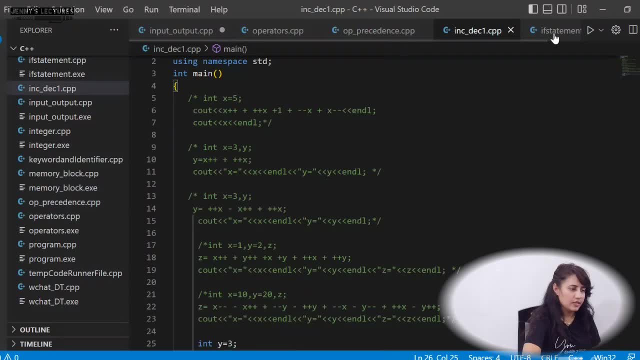 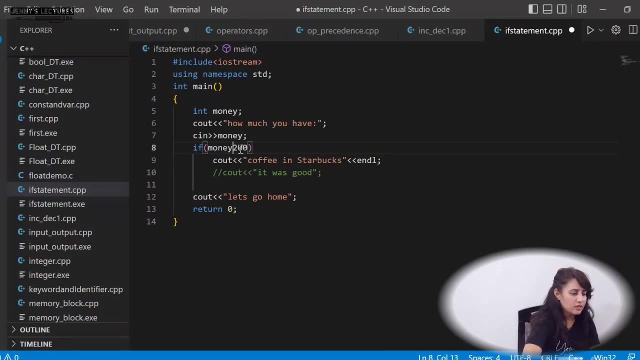 Right and in a sequence, and we will get the output. right now, we simply we are taking a variable into money- how much you have seen money? and we are checking the condition. if money greater than equal to 1000, then go in starbucks and just remove this line. let's go home, right? 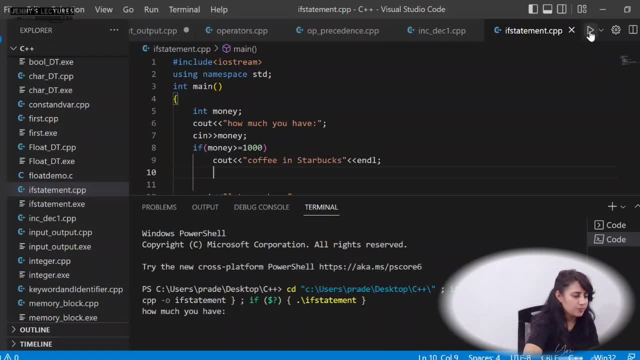 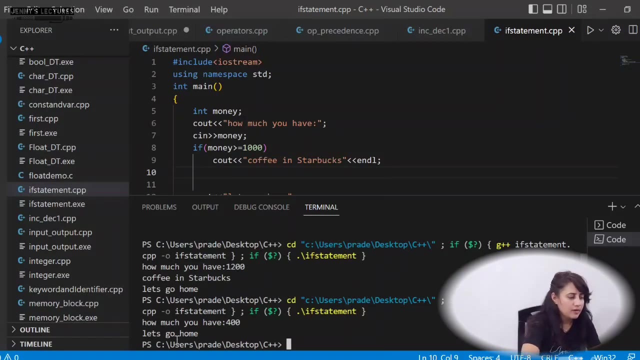 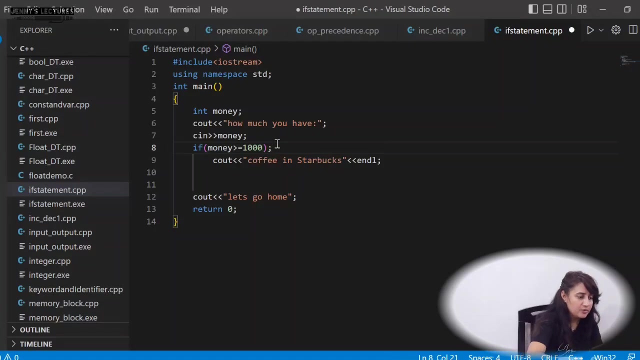 now let me just run this simple one first see. it will ask how much you have. i'm just entering 1200, so coffee in starbucks and let's go home again. if i run this and we have only 400 rupees, then let's go home. no coffee in starbucks this time, right? if now, see, let me. 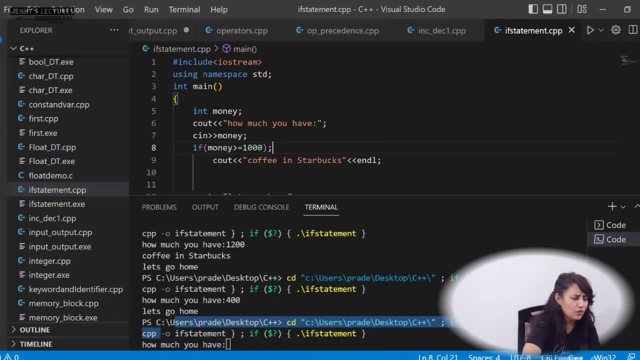 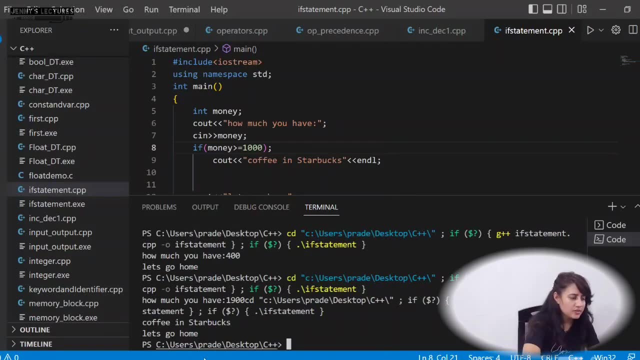 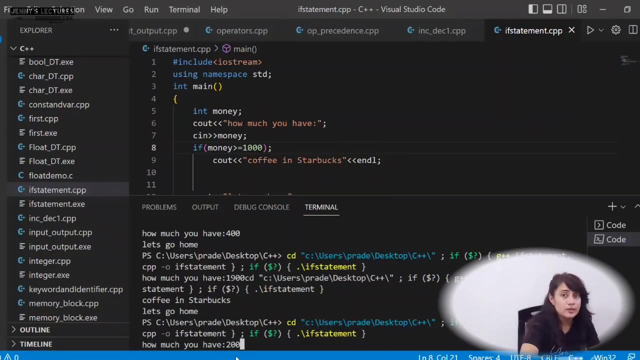 just terminate this line with a semicolon. now what output you will get. how much you have? i have 1900. let's just run this coffee in starbucks, let's go home, okay. fine, let me just enter now. i have 200. only this time condition would be false, but still it will print coffee. 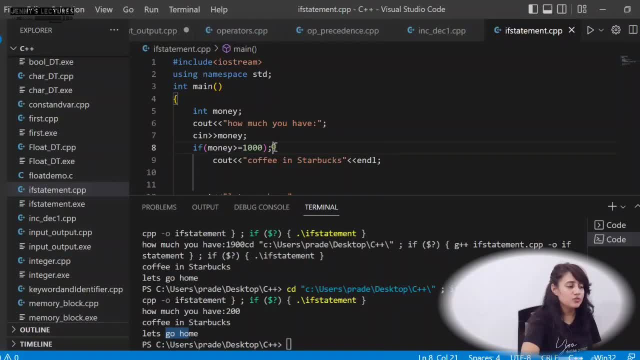 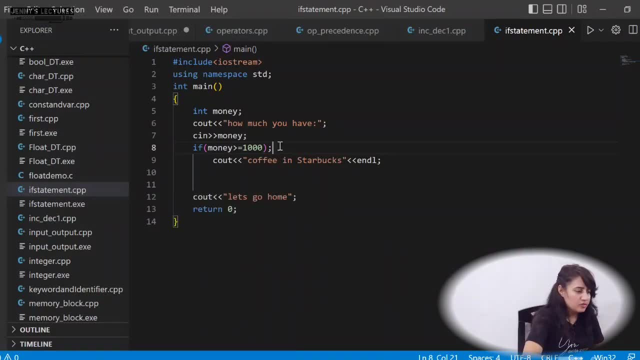 in starbucks, let's go home same output. why so? because we, you have just terminated this. if block means there is no use of checking the condition here, right? so this is the thing now. if i write like equal to 1000, equality, check condition, equal to equal to right. let me just run this. 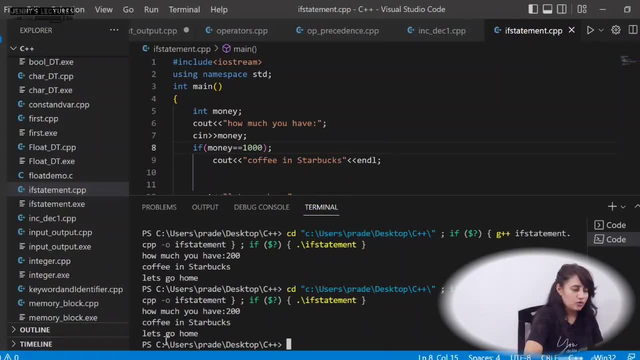 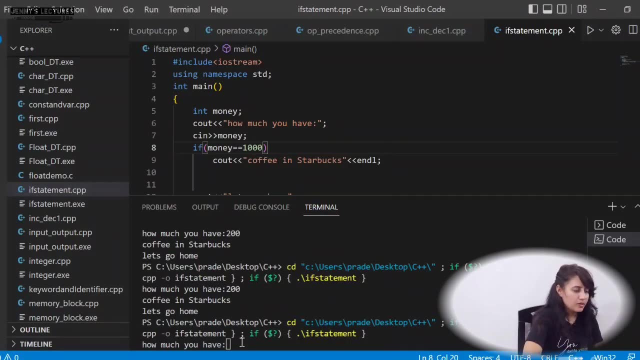 and how much you have 200 coffee in starbucks. let's go home. why so? because i we haven't removed the semicolon. let me just remove the semicolon. let's just run this again, see how much you have. now i have 200, let's go home. right, let's run again how much you have thousand. 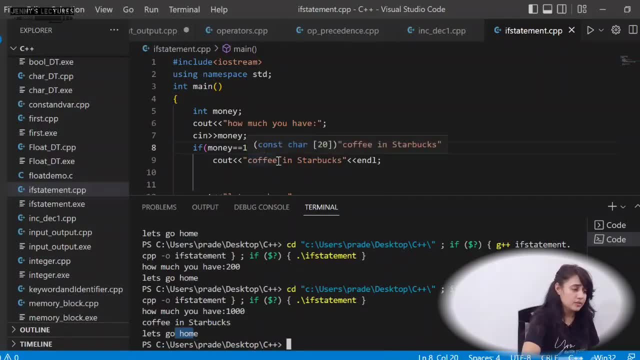 coffee in starbucks: let's go home right, because this time condition is true if simply, rather than double equal to, if simply i write equal to. but this is assignment optator this time right. so let's run this program again. 200 coffee in starbucks: let's go home right again: 1200. 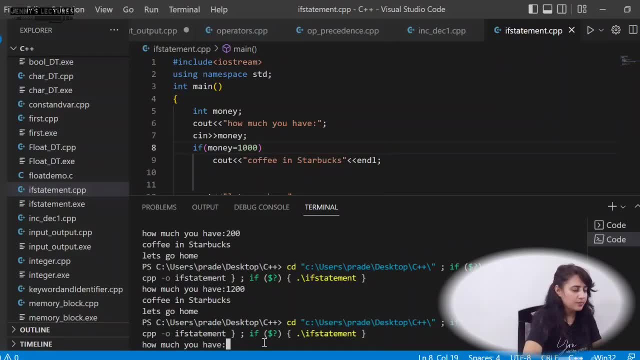 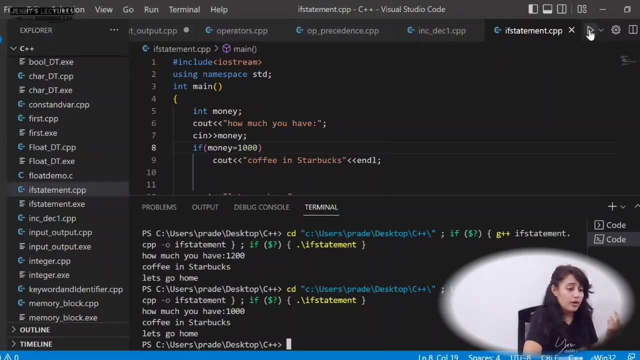 coffee in starbucks, let's go home. same output again: thousand of in starbucks. let's go home, because we are just entering. see, suppose i'm just entering zero. i have zero money. still coffee in starbucks, let's go home. why so? because you are just putting assignment operator here. it will simply assign the value. 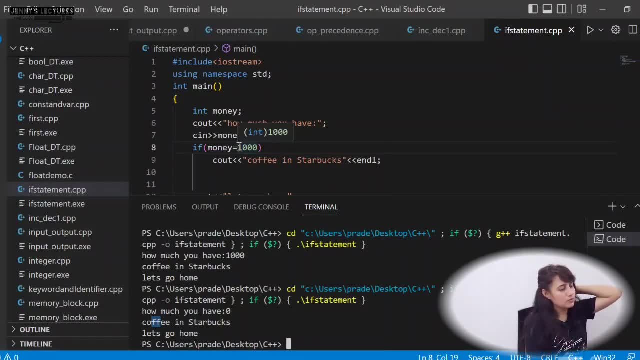 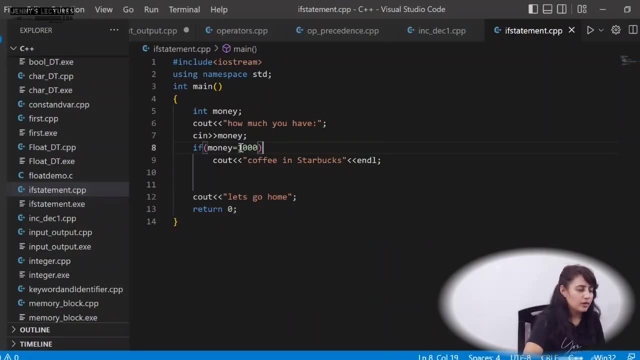 thousand to money, and that would be obviously all the time true other than zero. everything every other value would be true. so this you need to take care. equality check means double equal to now here, same condition. you can write down like relational operator. you can use logical operator, logical and if you want to combine two statements, right. if you want to find. 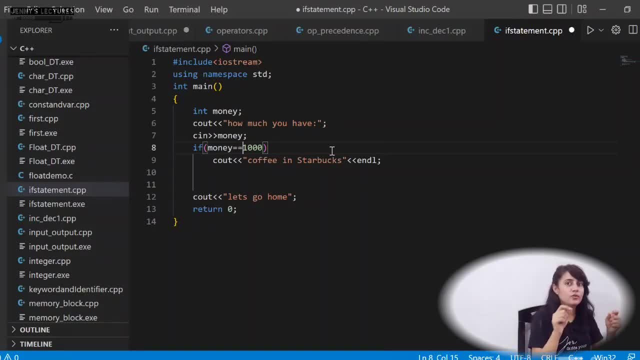 out like maximum of two numbers: a greater than equal to b and a greater than equal to c. maximum is a, this kind of thing. so you can combine logical and logical or these kind of statements. logical, not also right, relational operators, multiple statements, multiple conditions. you can write. 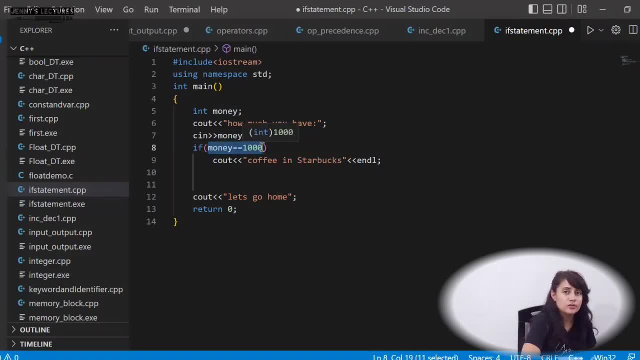 down this. if it's not like that, you can check. only one condition: right, like money: i am writing money greater than equal to thousand. right, and and one more variable: i am taking age greater than 15.. one more value, one more variable age we are taking and simply see out. 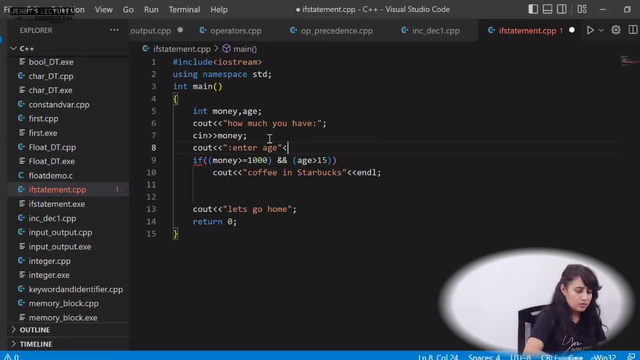 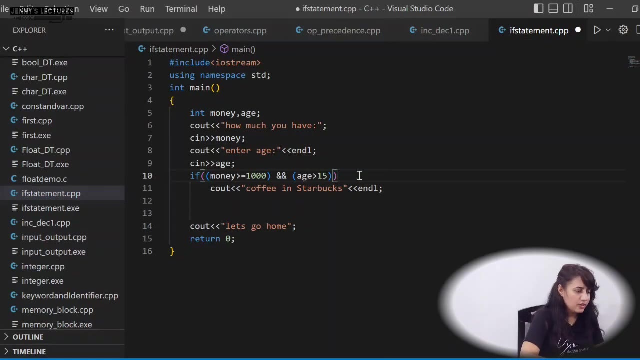 enter age. right, we are just entering age, that's it right. so now, yeah, we know there is no age bar. when you go for a coffee, it's no interest level somewhere else. but let's take a simple example. i'm just combining two conditions: money greater than equal to thousand and age should be greater than 15. then only you can have. 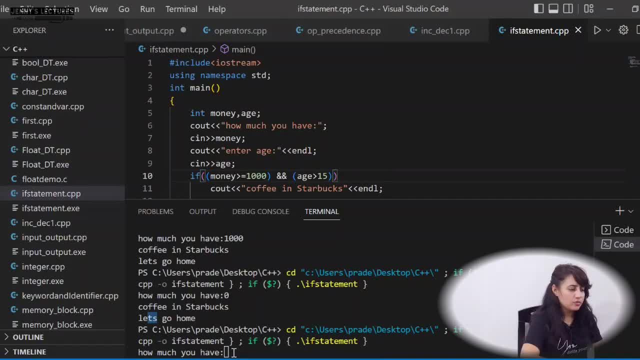 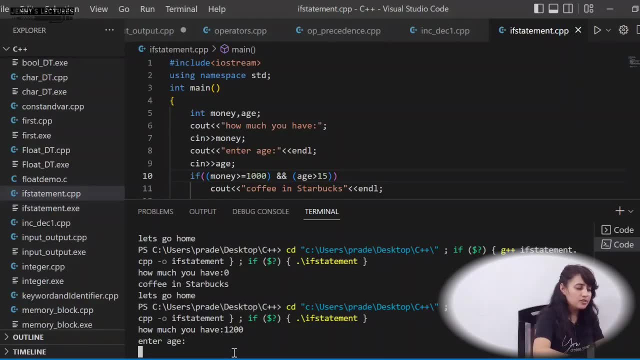 coffee in starbucks. otherwise, let's go home now. let's just run this. first it should ask how much you have money. yeah, money, i have 1200. then it will ask age. suppose you are entering ages 10. let's go home. no coffee in starbucks. 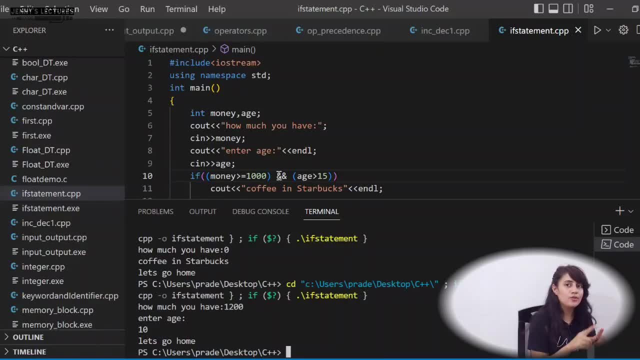 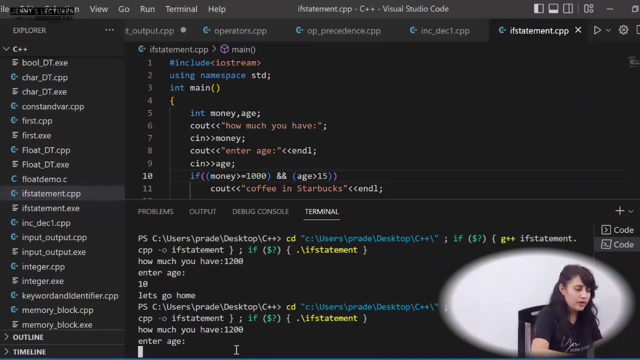 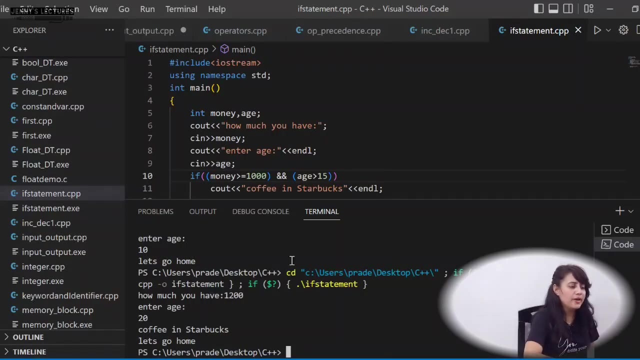 means both the condition should be true, then only it will be evaluated as true, right? let's run this again: how much you have 1200, age 20: now you can have coffee in starbucks, let's go home. so simply, i just want to, you know, tell you this thing: you can combine two, three, four conditions in this. if 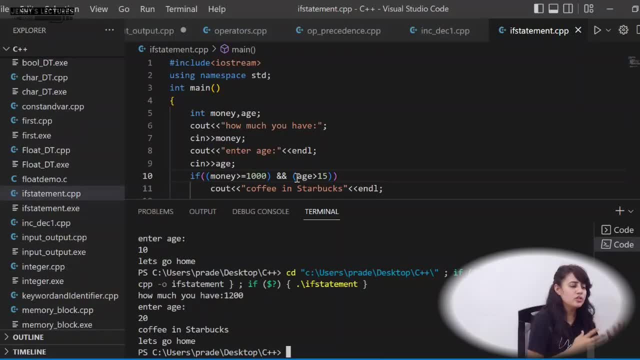 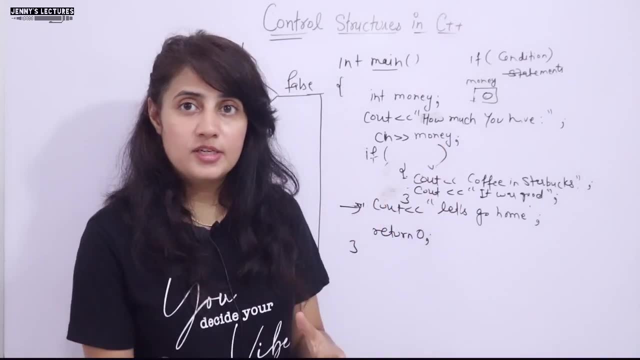 also logical and logical or operator you can write down so you can try out these combinations also. right? i hope that's it for this video now. so if you have any doubt in this, if blog, you can ask me in comment section, or if you you try out different, different things with this, if blog, it's not like.